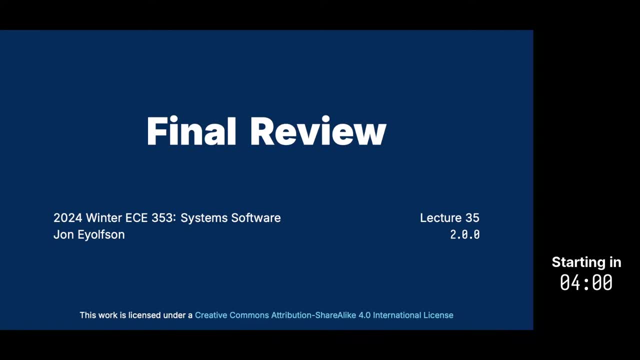 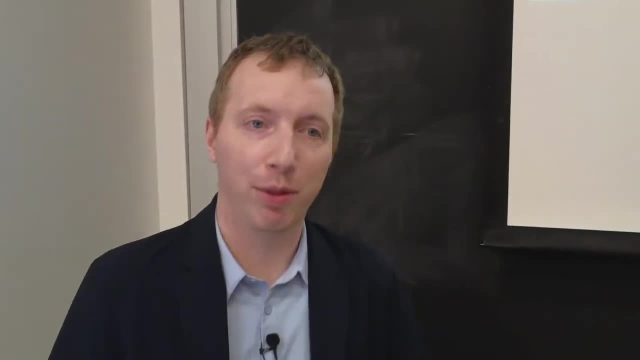 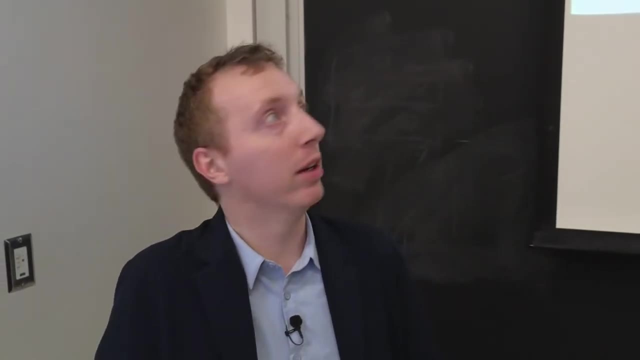 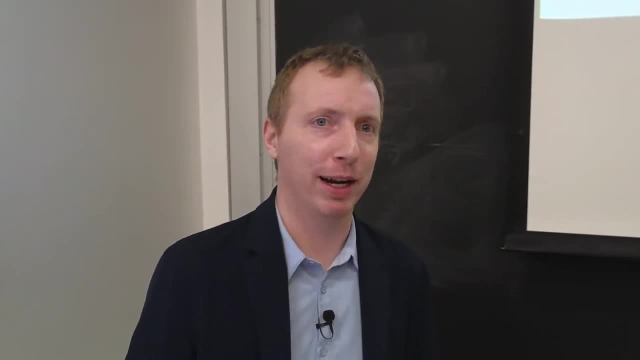 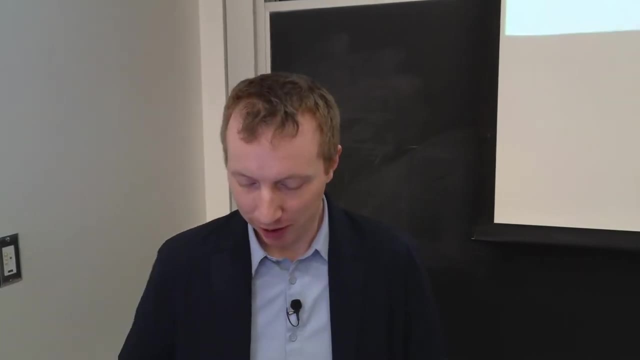 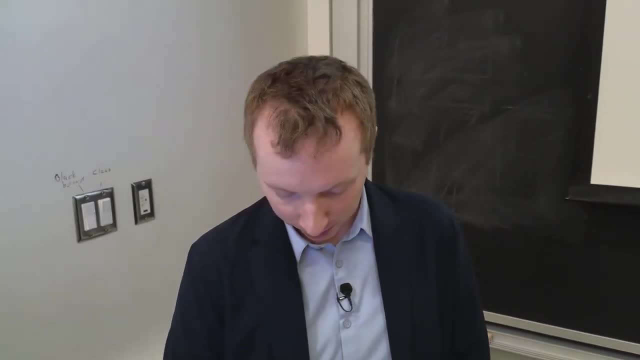 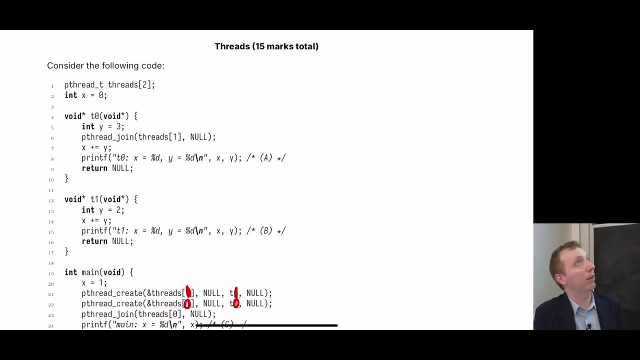 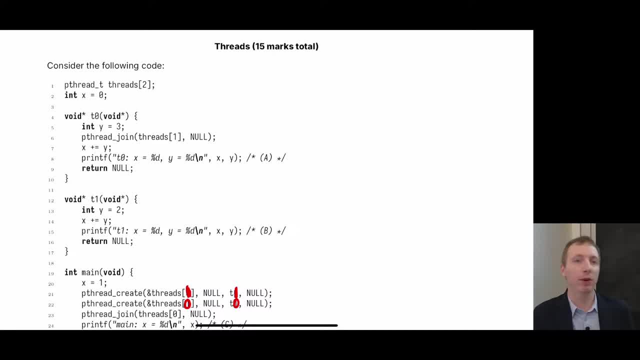 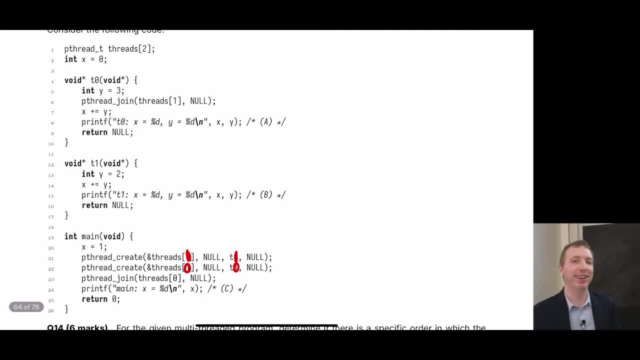 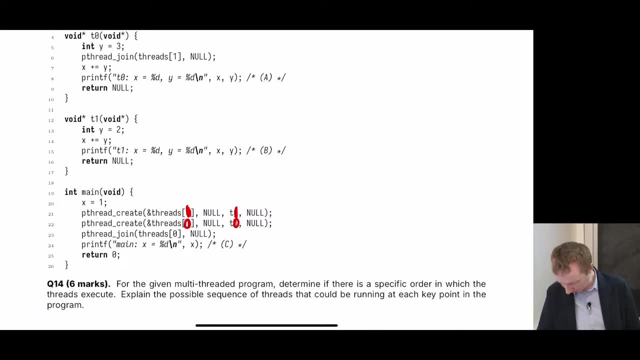 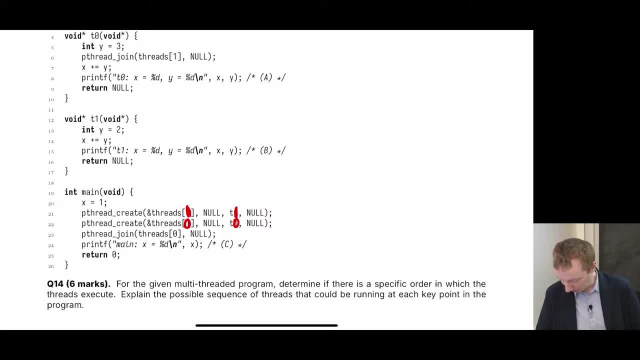 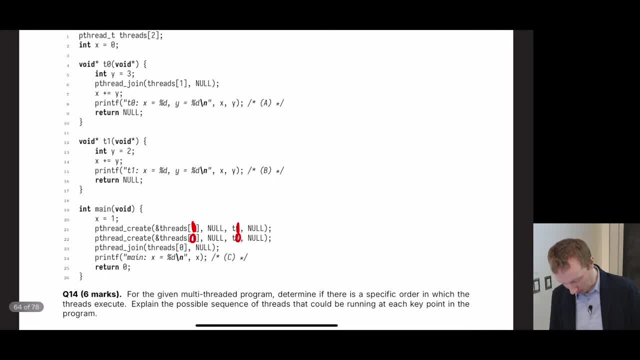 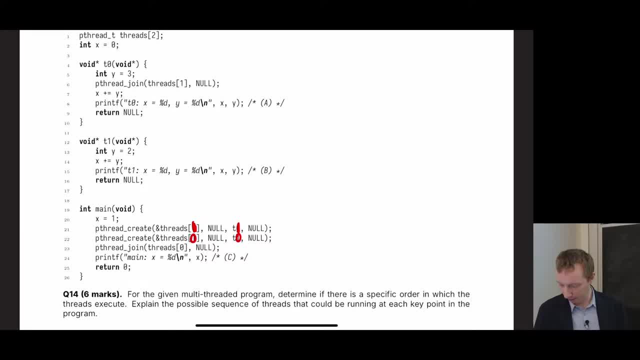 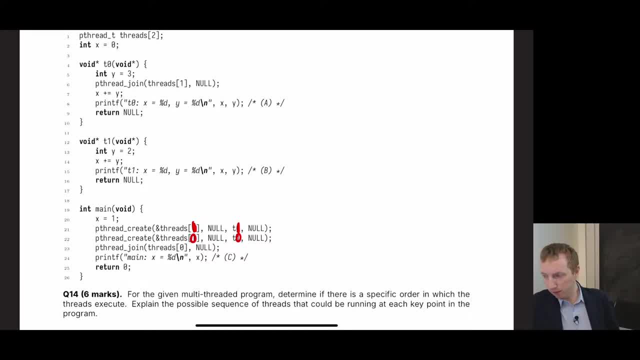 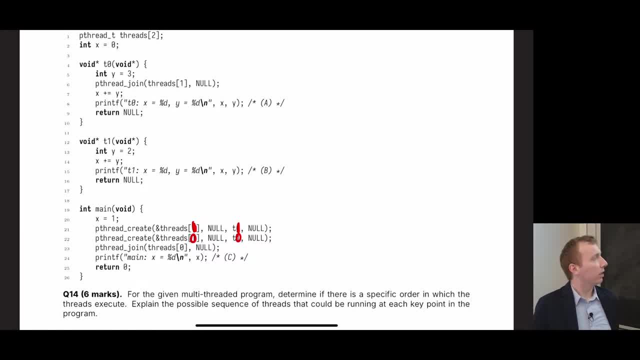 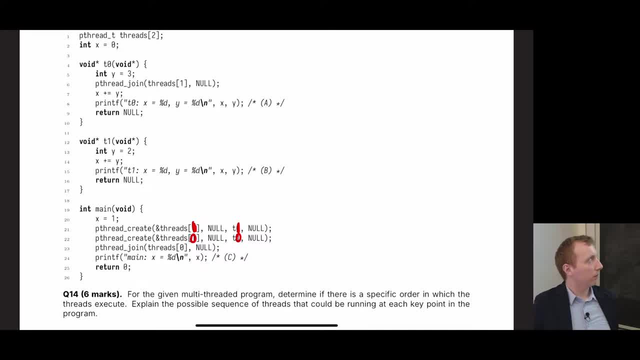 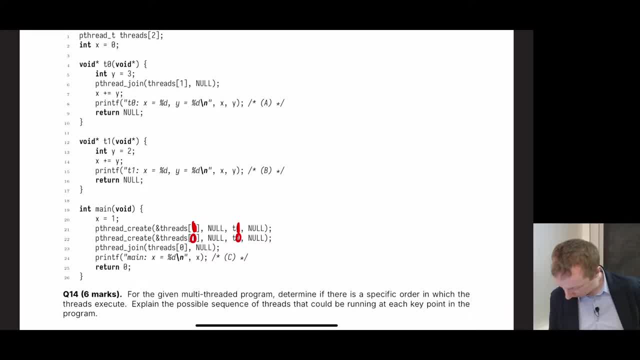 Yeah, so there's going to be a specific order, at least how it's written right now, because, well, let's see, I'll put it in blue. We have our first main thread running. It would set a global variable to one. 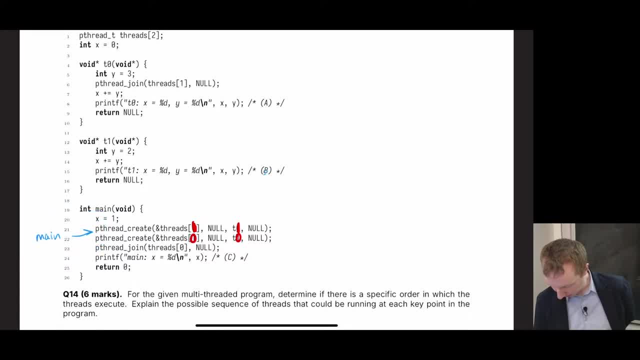 then create thread one. Now, at this point we don't know which of of these two could run. So could be the case where thread one runs all the way to completion, Could be the case where main goes next. We don't know. 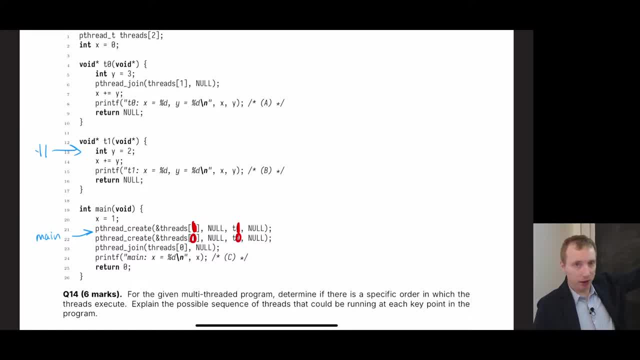 In this case, nothing's stopping thread one from finishing right now. It could just go right to the end before we even create thread zero. So no specific order so far. Then main creates thread zero. So that would start off like that, And now any of these could run. 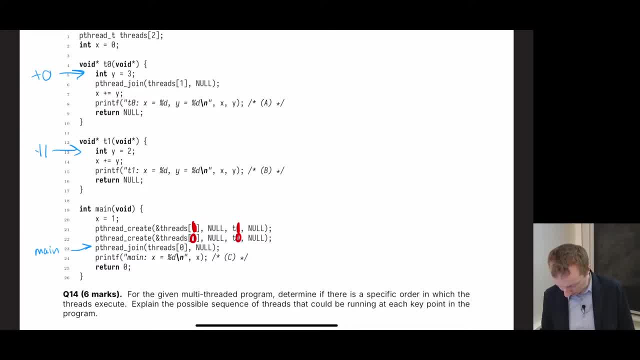 But well, if the main happens to run, it's not going to get that far, It's just going to make it to join And it can't make any progress until thread zero is done. And then thread zero. well, it can set its own local variable to three. 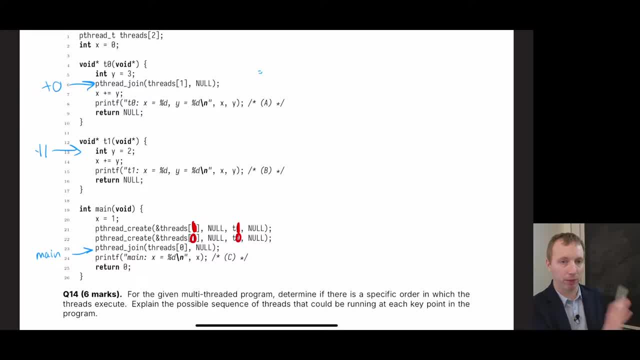 and then join. And now, at this case, we have no choice but to execute thread one, right? So there is a specific order. We have to execute thread one first. We have to execute thread one first. It has to complete first before. 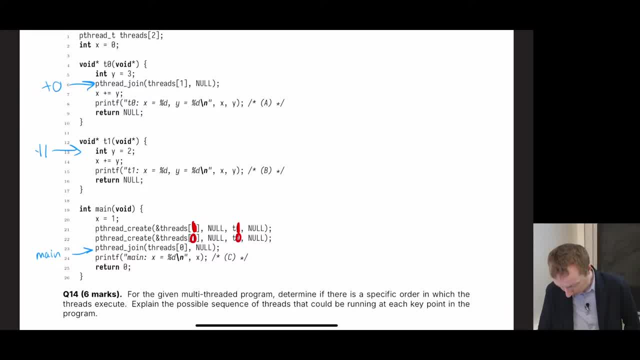 So thread one has to complete first before thread zero passes line six. So thread zero cannot pass this line before thread one's done, And also the main thread cannot pass this line well, before thread zero is done as well. So no choice but to actually execute thread one. 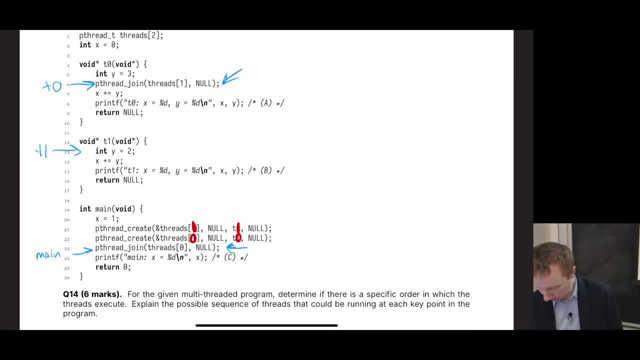 in this case right. So is a defined order Thread. one has to finish first, So it would create. it has int y, So int y local variable to thread one, Then y is equal to two. It would increment the global variable x. 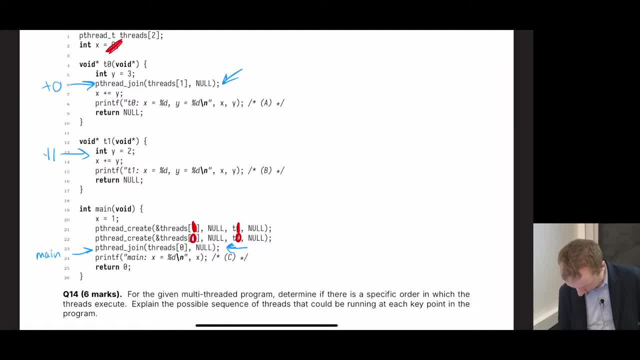 So here I'll write out what x should be. So the main thread updated x to be one whenever it first ran, And then now we increment x by two, So we should update the value to three Then. well, we've already done the first question, right? 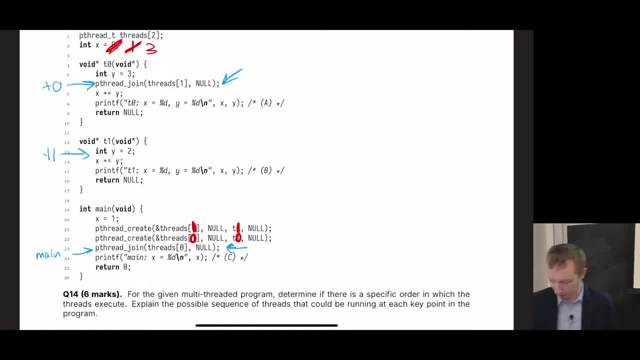 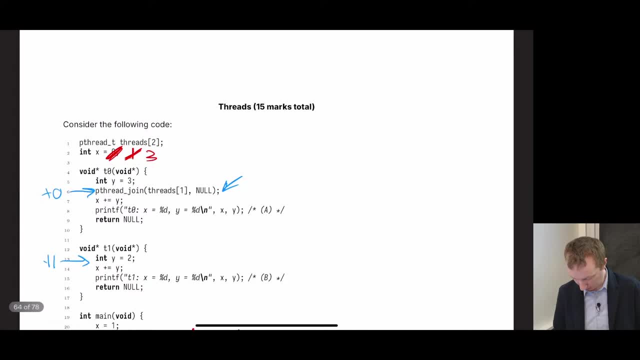 We just said what the order is and they have to run in this order. So now we're doing the next question. that says identify all possible outputs of this program may generate when executed. So right now we can only execute thread one, So we're doing that. 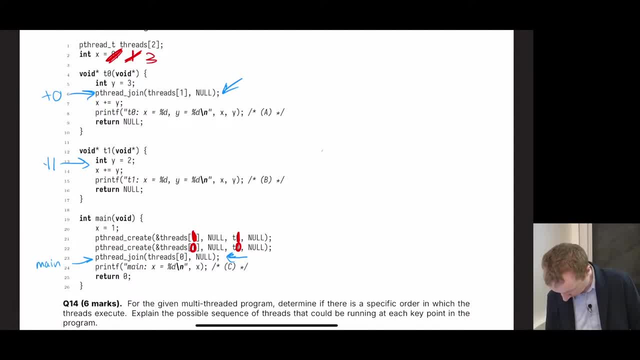 So now thread one would print off thread one, And then we're going to print off thread two, And then we're going to print off thread three, And then we're going to print off thread four. x equals three, Y equals two. 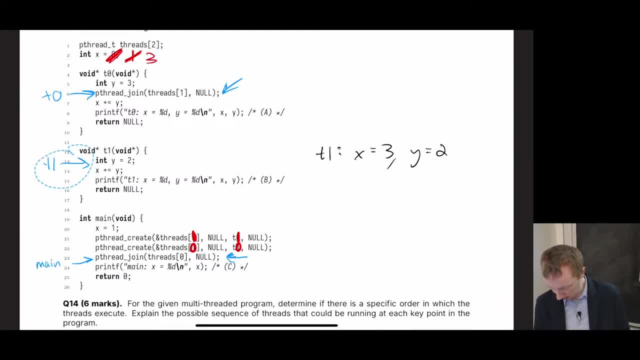 And that's it right. Then thread one is done. And now, since thread one is done, the only thread that can run now is thread zero, because it can now return from the join, because thread one is now done. right, So now thread zero is the only thing that can go. 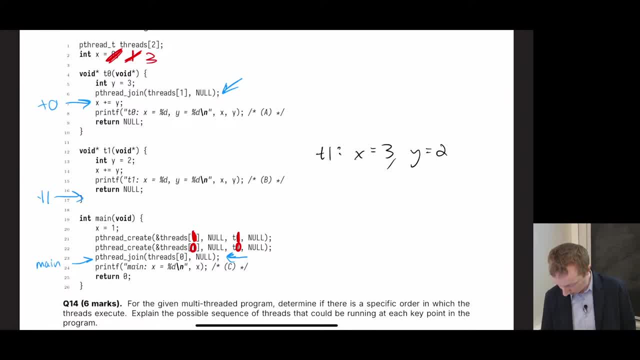 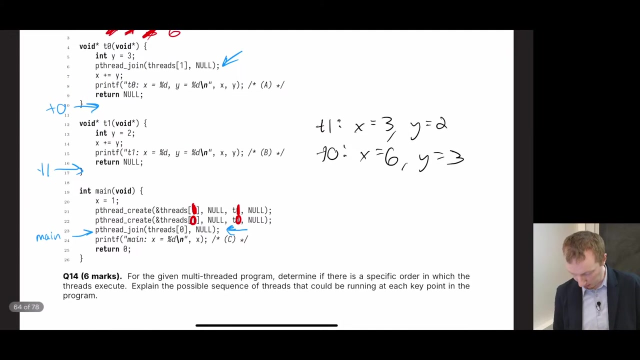 It increments the global variable x. X plus equals Y, which its Y is 3, so we increment it to be a 6.. Then it prints off thread 0, X equals 6, Y equals 3, and then it's done. 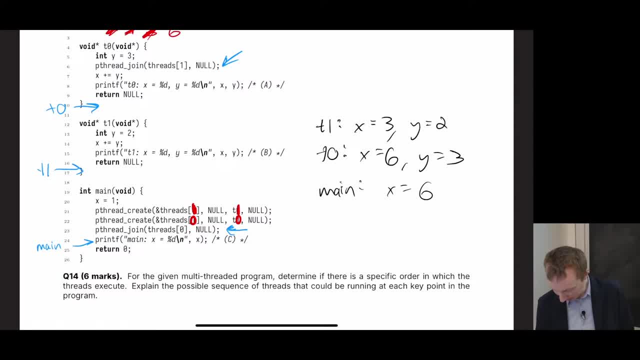 I revised it because I looked at them like you know what, having it say 1 then 0 looks a bit silly to me. I think it would read better if it was 0 then 1.. So I just did this and then gave that as a question. 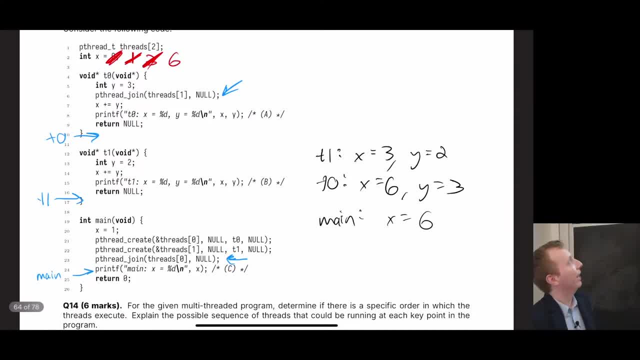 So this makes it infinitely harder. Anyone want to explain what happens if I do something silly like that? Yeah, Like you could essentially be trying to join a thread that doesn't exist. Yeah, I could join a thread that doesn't exist, So I could create thread 0. 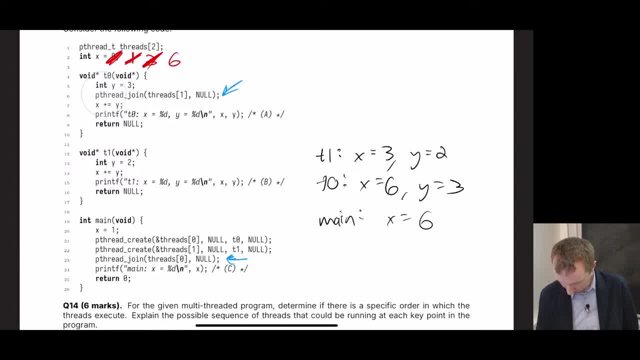 So here let's rewind all the way back. So I start with my main thread again. I update X to be 1.. So now instead of 0, it's a 1.. Then I create thread 1, or, sorry, thread 0.. 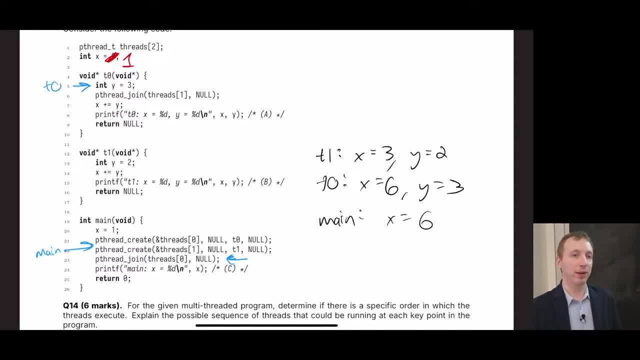 And if I create thread 0, now I don't know which one executes. So it could be the case That thread 0 executes, So it would create its own local variable Y, which is fine, But then it would join thread 1, which doesn't exist. So it would just get an error. So it would just return immediately, like in your lab 6, or, sorry, lab 4.. It would just probably return negative 1, be like that thread doesn't exist yet. What are you doing? 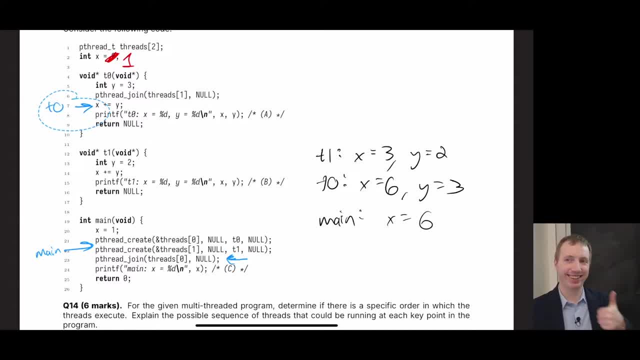 And then it can just start executing now And then the amount of data, But the main is part of the output. It's a different output that it generates. So now, in the case that you print thread 1, you can print thread 0. 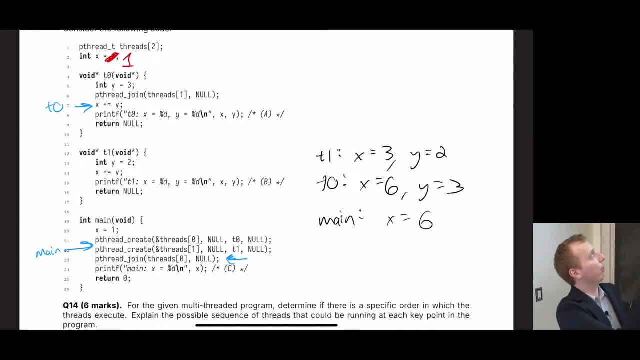 And then the output comes in. you know different outputs you could get, So you could still possibly get this output, But you're not guaranteed to So now, in the case that Join just returns an error, it just keeps on going. I could print thread 0 first. 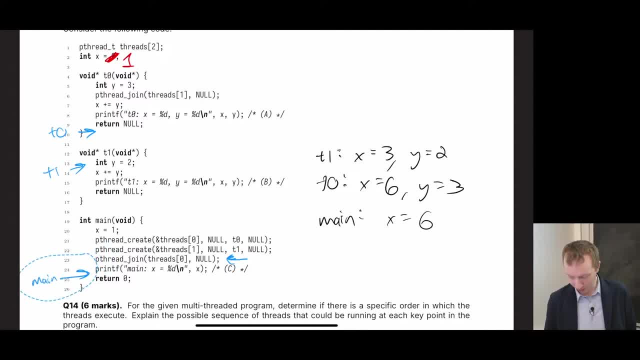 And then thread 0 can be done, Then I could join on thread zero and then print main, and then I can print thread two and like there's so many different output possibilities here that yeah, oops. So for this I like made this worth five of the six marks. 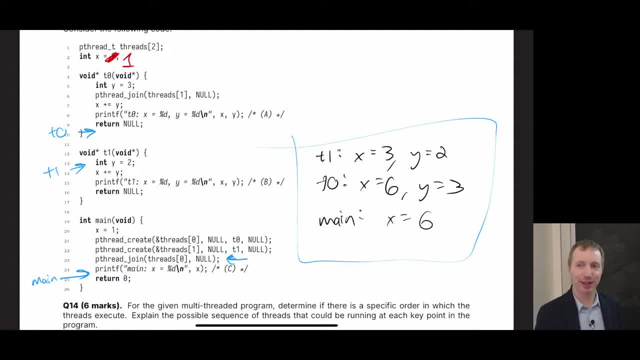 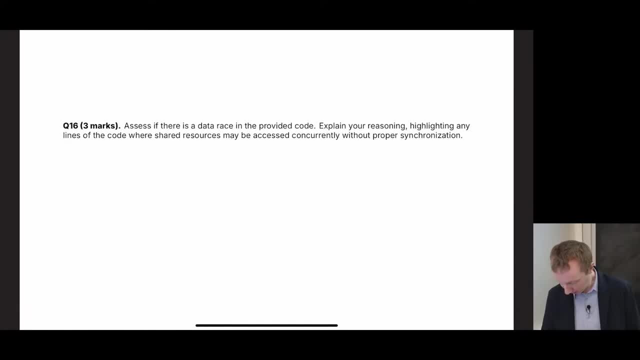 And then if you said any other possibility, I gave the other mark as a way to like oops. sorry, didn't mean to make it difficult for you, But then it says: assess if there's a race condition. the provided code explain your reasoning highlighted any lines of code where a shared resource might be accessed concurrently without proper synchronization. 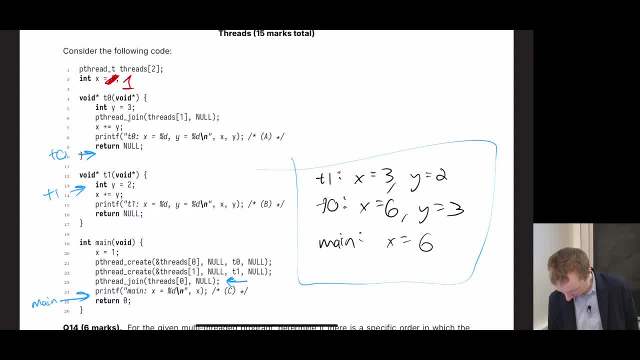 So if we rewind a bit, So in the intentional way, was there a data race? No right, They were all updating the same Global variable. Yes, but only one thread could have updated it at a single time. Therefore, we don't have a data race, because the data race is: we have to have two possible concurrent actions to the same memory location, with at least one being a right. 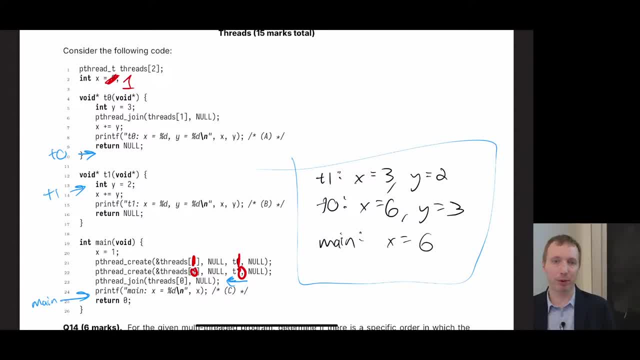 So it doesn't happen in this case at least. So we're all good. In the other case, definitely happened, So you could just say yes and just say what the data race was, because join has an error. All right, Are we all good for that question? 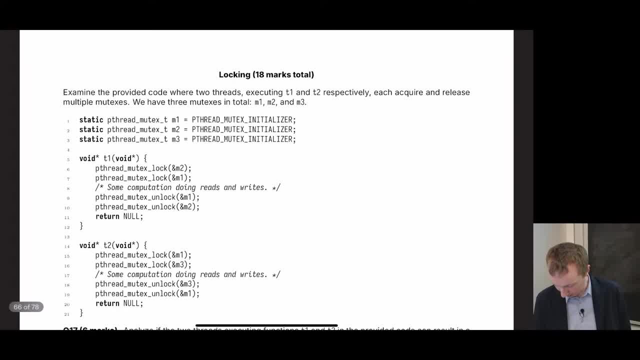 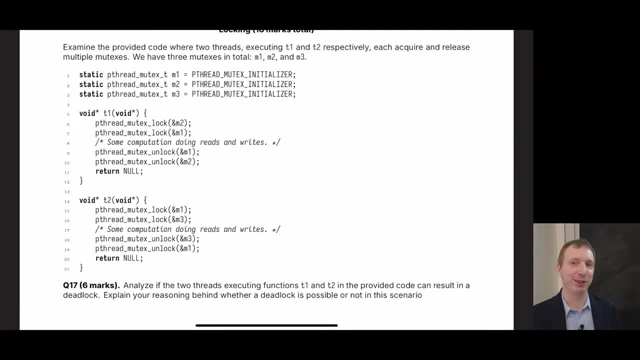 All right, Other fun questions. So the other one was synchronization. So, Oh, I heard a groan already. Yikes, All right, So there will definitely be synchronization on the final. So it says: examine the provided code where there's two threads. 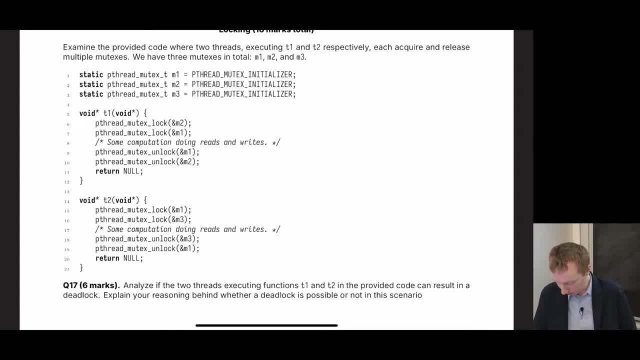 They're set up to execute T1 and T2 respectively. So we have two threads set up. They're set up to execute these. that says each acquire and release multiple mutexes. say we have three mutexes in total and one and two and three. first question says: analyze if two threads executing functions- thread one and thread two, in the provide code can result in a deadlock. 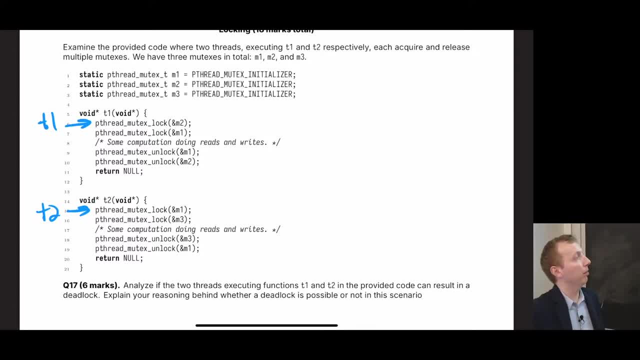 Explain your reasoning as to whether or not a deadlock is possible or not in this scenario? Yeah, I don't think so, because the only mutex lock that's between these two is M1, and M1 can't be locked permanently without the other one. 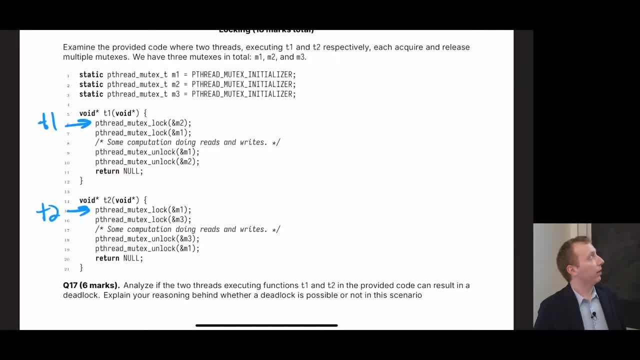 Yeah, So with this, Two different ways you could explain it. First, that the only lock that's shared between them is M1, and neither thread is trying to acquire another lock the other one has. So there is no possibility of hold and wait, because, well, I'm not. 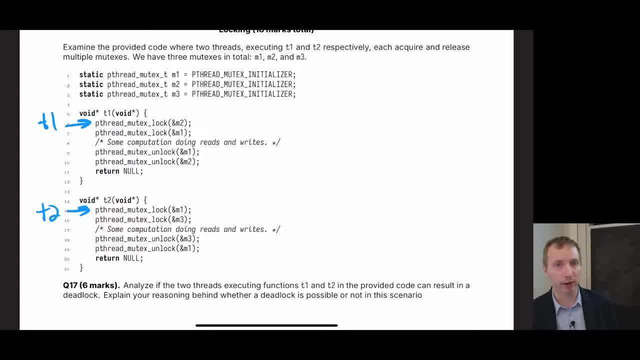 trying to get a lock that another thread has. and also there is not any circular weight here either, right? So T1, while it has M2, it just wants to get M1.. If T2 tries to get M1, it wants to get M3.. It's not a circular weight. I can't draw a. 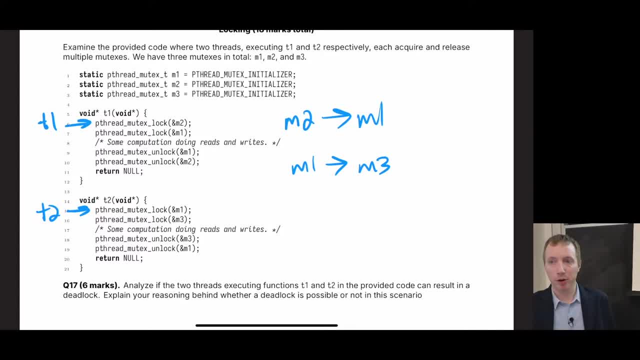 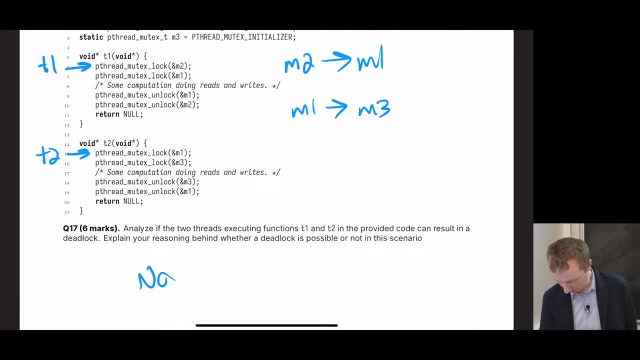 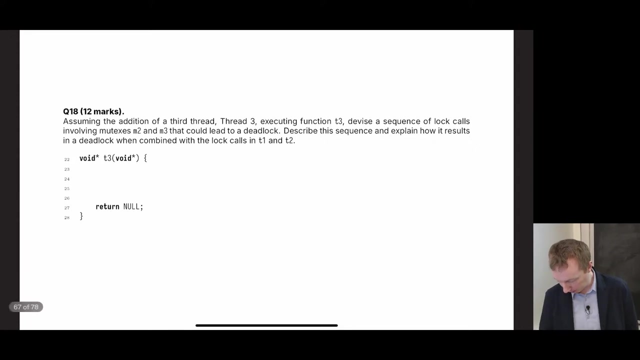 circle between all the dependencies. so no possibility of a deadlock here. So could say either, just if you want to do this really short, short, No circular weight, Boom, Six marks, How easy was that? eh, Then it says: assume: addition of a third thread, thread 3, executing function T3.. Devise a sequence. 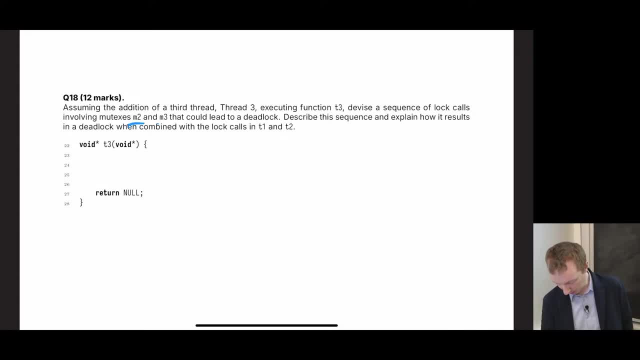 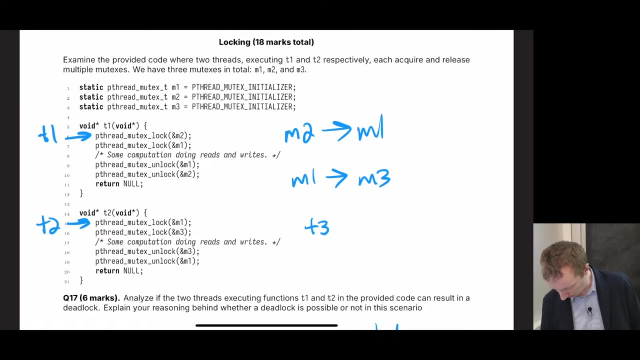 of lock calls involving mutexes M2 and M3 that could lead to a deadlock. Describe the sequence and how it results in a deadlock when combined with T1 and T2.. So we want to create another function: Oops, Void T3. 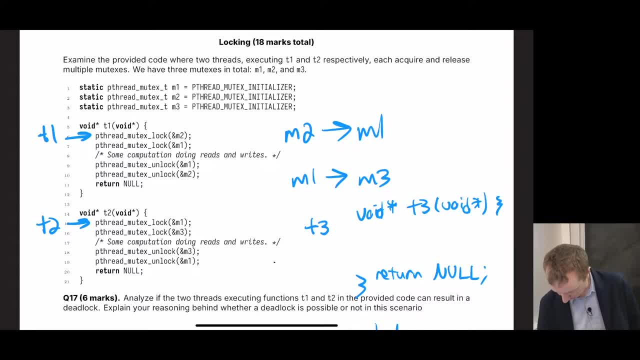 That somehow uses M2.. Then it uses T3.. Then it uses M1.. Then it uses T2.. Then it uses M2.. Then it uses M2.. Then it uses M3.. Then it uses M4.. Then it uses M5. 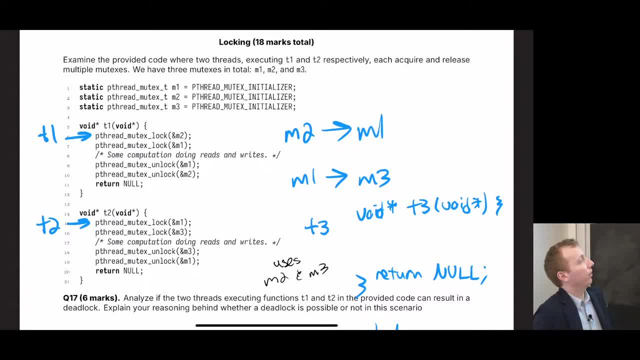 Then it uses M10.. Then it uses M11. and M3,, such that we do have a possibility of a deadlock. Yeah, You could do something where it's like you could have these guys lock M3, and then lock M2, and then do that. 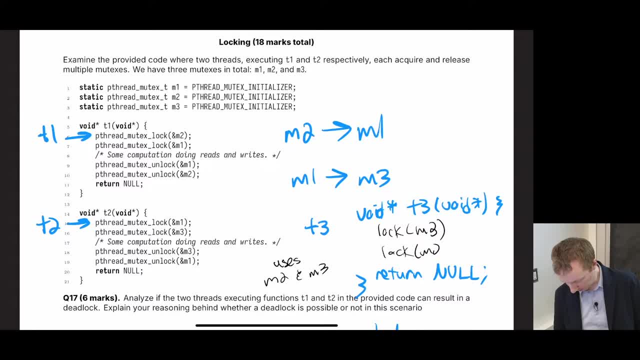 Lock M3, then lock And then like it unlocks, Yeah, and then I could, so I don't really need. you could unlock and be good, but we're just doing a deadlock, so we can just leave it at this. 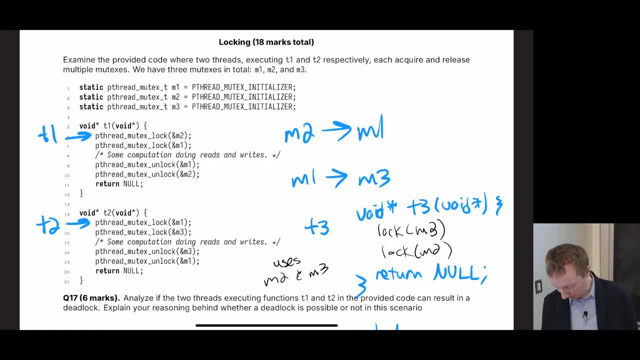 So if I have those sequence of calls, I have now created a circular dependency, right, Because now I have M3 that needs M2. And now if I add that to the other two, well, there's my circular dependency. 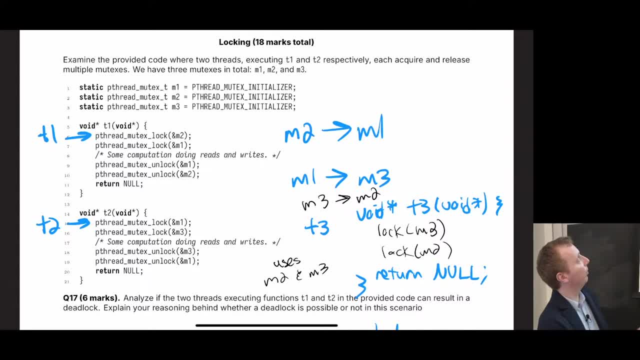 So I could run it: thread one gets M2, and then we switch to thread two, it gets M1, and then we context, switch to thread three, it gets M2.. So and then, yeah, thread three gets M3,. 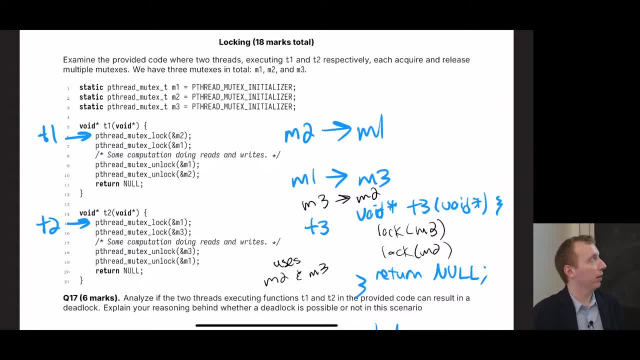 and then we're screwed. No thread can make progress anymore. therefore, we are now deadlocked. So I tried to be creative here and flip the deadlock question to, like you, make a deadlock instead of: is this a deadlock? 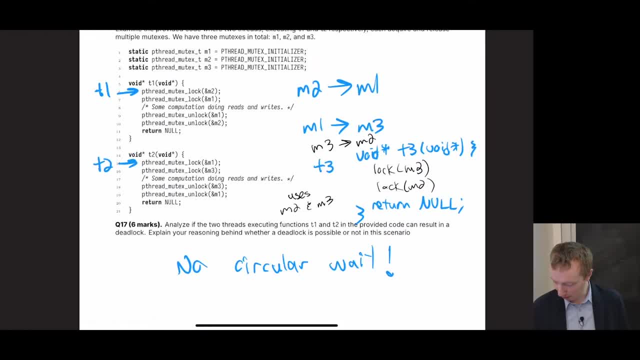 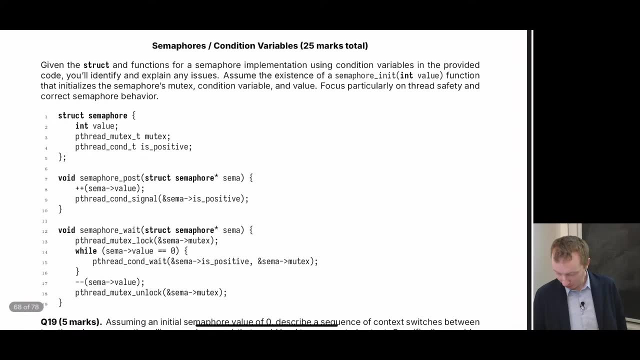 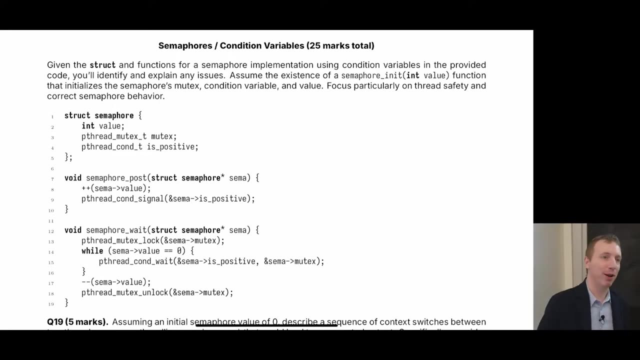 So wow, See, I don't know. I'm pretty much out of creativity, though, So we'll see what you get. All right, Next one: Wow, we are cranking through this. So that was, like most of the questions, the long questions. 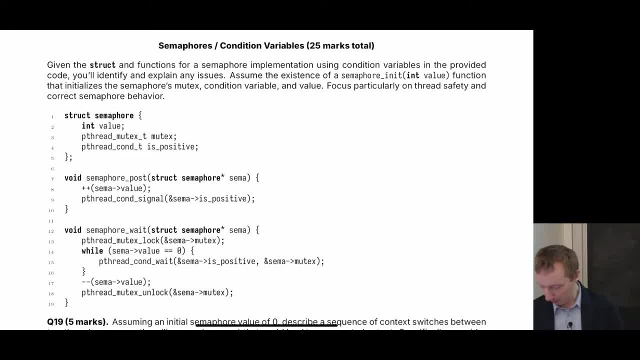 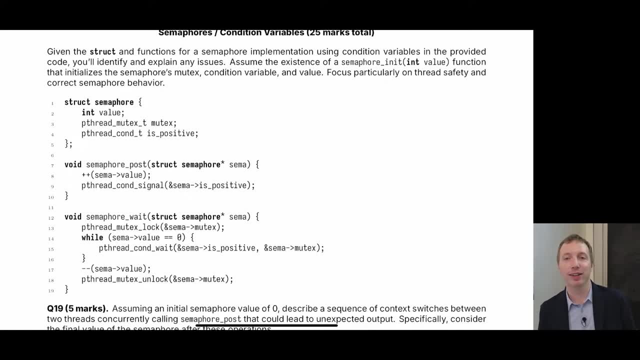 So we're almost done this exam in 15 minutes, So everyone should be able to go home early, right? Yeah, probably not. Huh, Is this like why exams get written to be like so long? 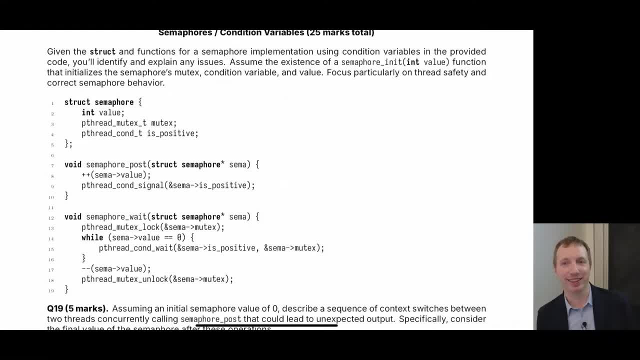 Because you're like looking through them and you're like, oh, this is amazing, Yes, Yeah. So typically to time an exam, I try it myself and take how long I took, multiply it by four or five. 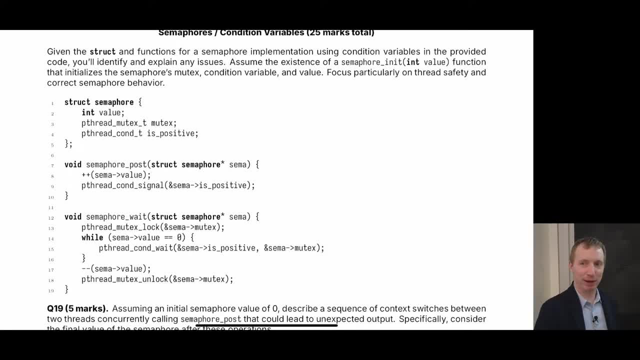 and then if it's under the deadlock, then if it's under the exam time, that's about right. So Yeah, I think I had to raise it. I think I started at like four and now I'm up to five. 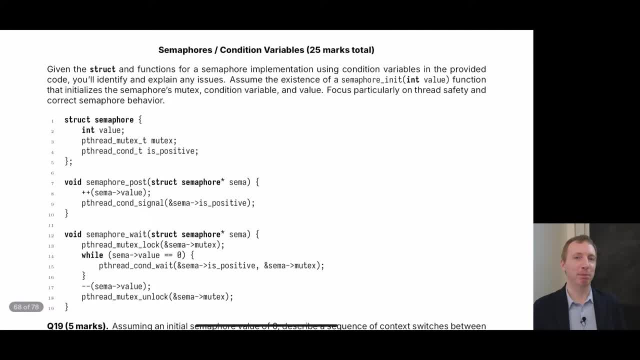 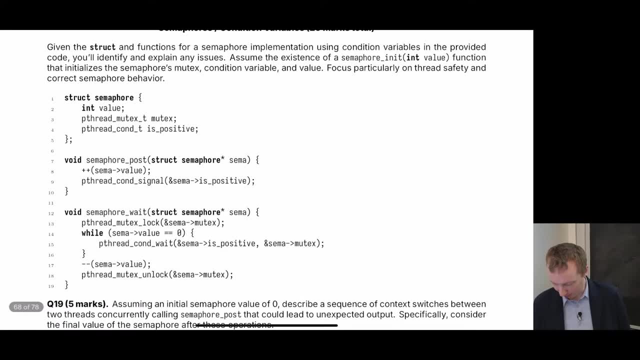 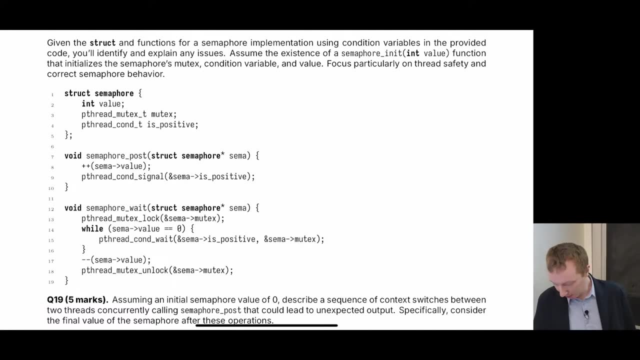 So that's the problem, right? I get better as it goes on, and you guys are a new class every time. so Yeah, so I'll probably multiply it by five this time, All right? So next question: Given a struct and the functions for a center for implementation, 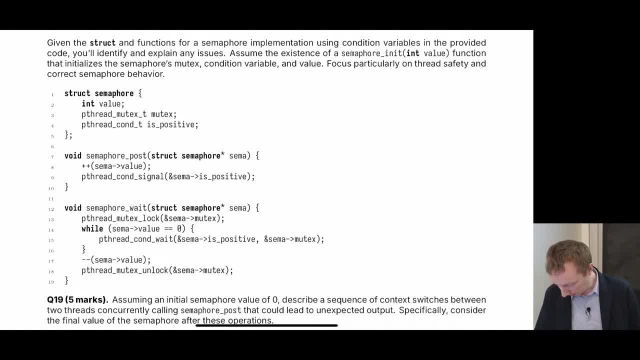 so we're trying to implement a center for here using condition variables. in the provided code you'll identify and explain any issues. Assume the existence of center for init value, that initializes the center for mutex condition variable and variable Focus particularly on thread safety and correct center for behavior. 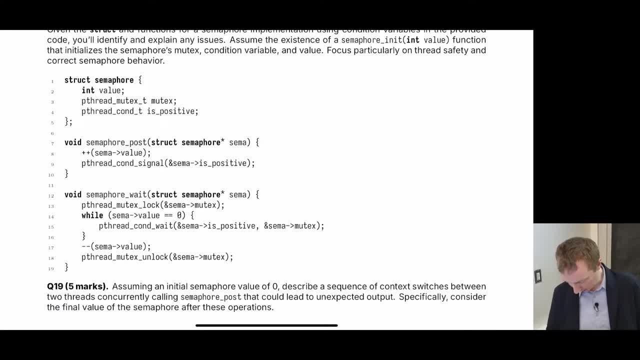 So first question says: assume that the initial center for starts with a value of zero. Describe a sequence of context: switches between two threads concurrently calling post. That could lead to unexpected output. Specifically, consider the final value of the center for after these operations. 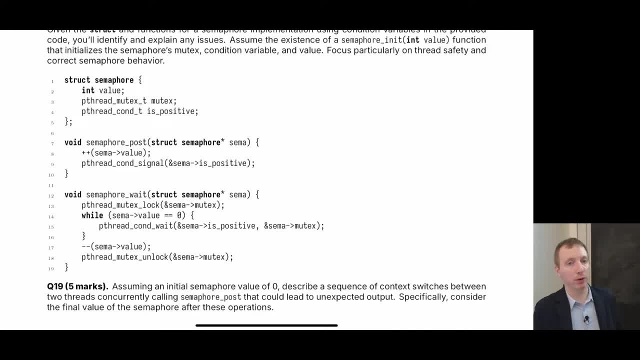 So I have Two threads trying to call post And for when these questions are set up like that, I had some students to say assume a call also happens to wait, and then they like randomly jumped in the middle of it. 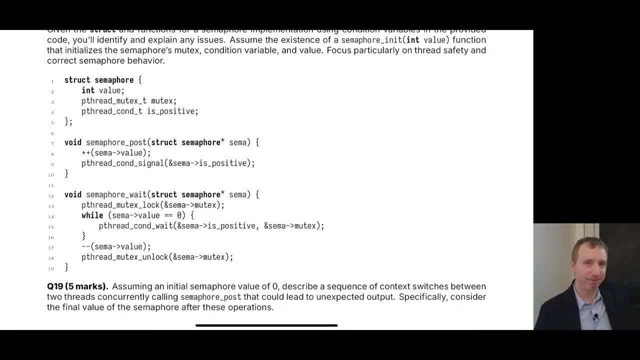 or something and didn't start from the beginning, And I can't give marks for things that are impossible. So please know that functions start at the top and go down And if the question says two concurrent calls with two threads to post. 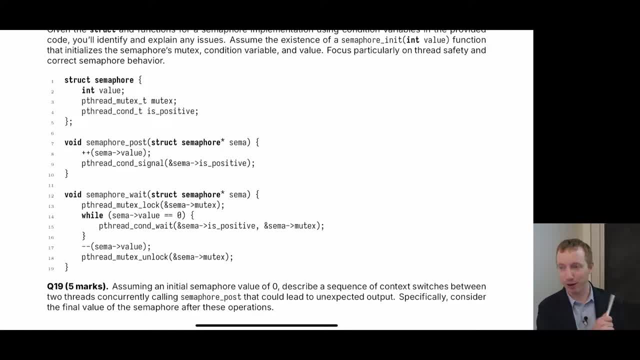 you should explain it in terms of two threads calling post. So we have thread one set up here, also thread two set up at the same place, So initial value is zero. and then if I have two concurrent calls to post intuitively, what should the final value of the center for be, if it worked correctly? 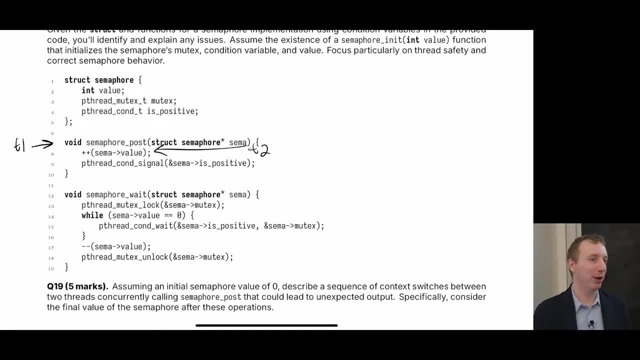 Two right. Two Starts at zero. Two calls to post. It should be two All right. So it says: is there a way two concurrent threads call post? that leads to some unexpected output, aka any output. that is not two. 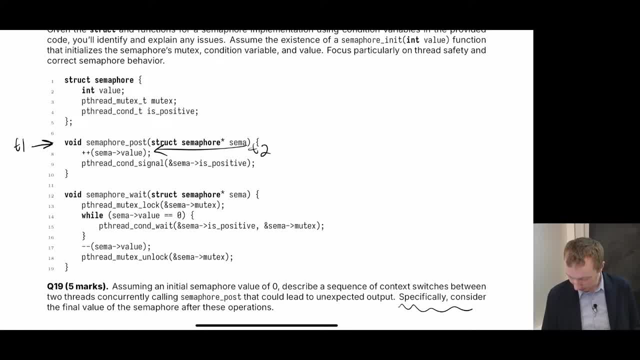 And then it even explicitly said: consider the final value of the center for So is there any way the final value could be zero or one? Yeah, I'm guessing it's going to be one. And if they both get called at the same time, then that summa increment or the value increment. 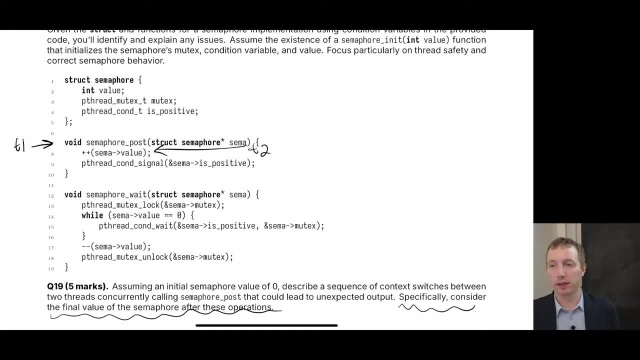 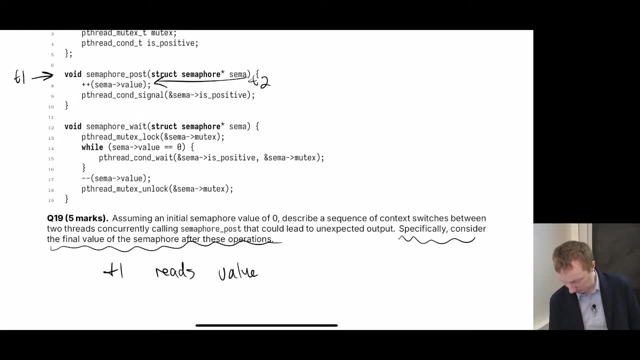 that's not atomic, So one could read it, then the other one could read it, and they can both write it at the same time. Yeah, So plus plus not atomic. What may happen is that thread one reads value zero. 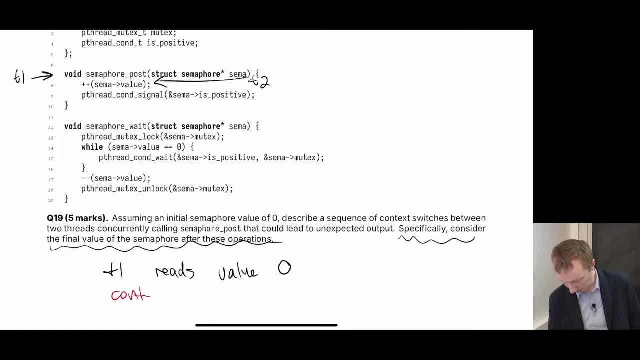 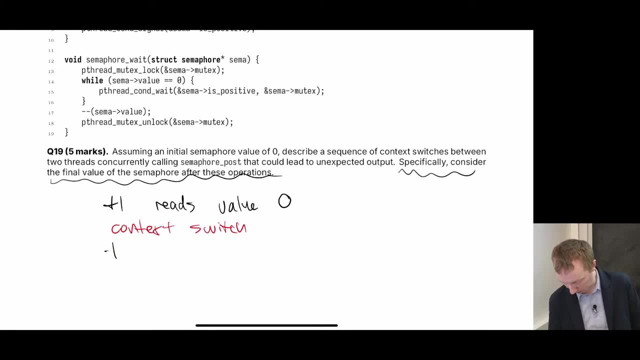 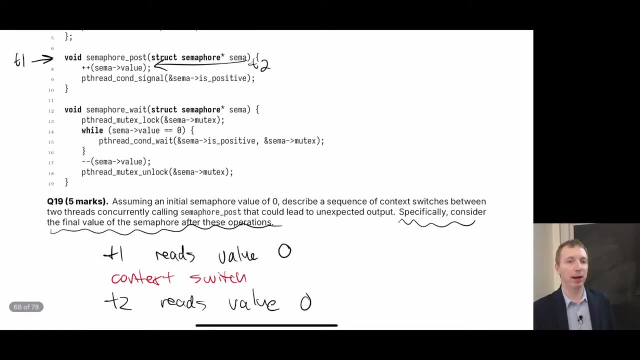 You can even do it in red Context switch. Then now we're running thread two. It now reads a value of zero, And now doesn't matter what happens. right, They're both going to update it in the registers, which are independent, and then write the. 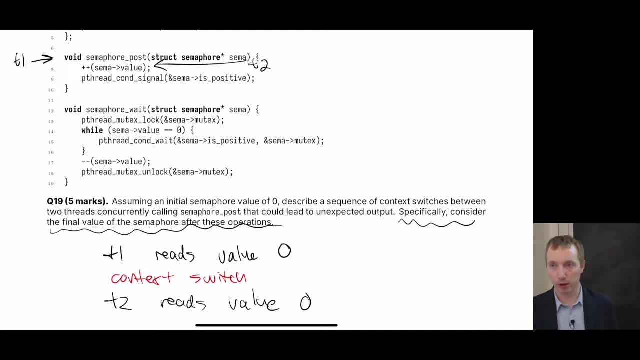 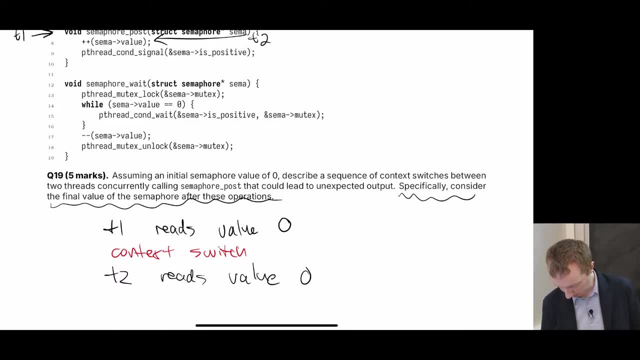 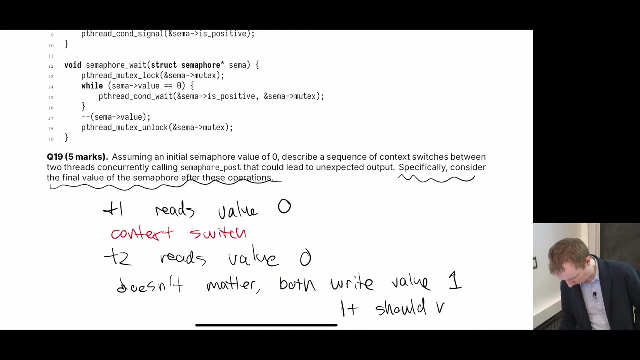 value of one to that location, so the final value is going to be one Then. Oops, Then. Well, my writing's bad Doesn't matter. Both There, That's all you had to write, So we have a switch. 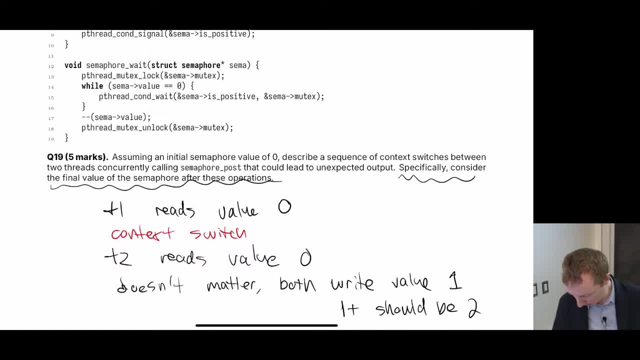 As soon as they both read zero, then we're screwed. They're both going to write the value one, Then we get the final values. one should be two. So everyone good with that. All right, I can already guess the next question I'm going to ask. 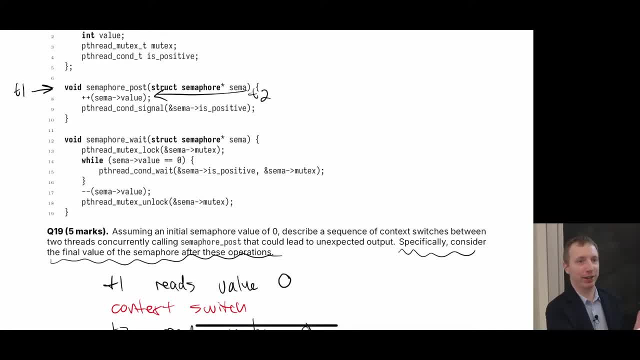 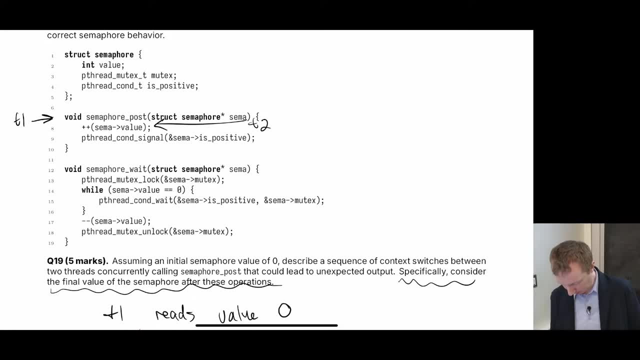 You probably should be able to too. Fix it, Yeah, Add a new text around the plus plus summa value and the condition x, the condition summa, as well. Yeah, Yeah, Yeah, Yeah, So, Oh, actually. 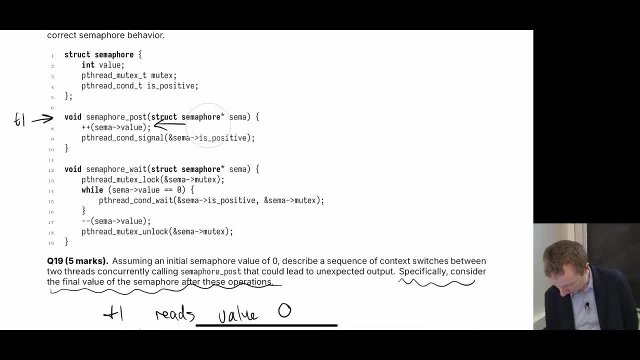 Yeah, So Well, if I was to fix this right, I need a lock before I update it. Do I need the unlock after the signal? Maybe after the increment? So Unlock, Yeah, So I could put the unlock after the update or after the signal. 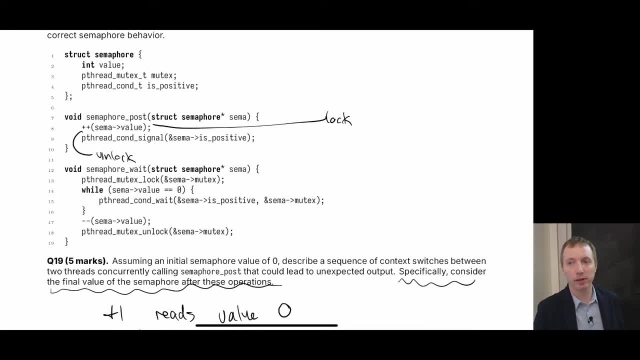 It doesn't matter. Both are going to work fine. What is the condition of the signal? Would that block if it was negative? No Signal just wakes up one thread that's waiting for the condition to change. Ah, Okay, Yeah. 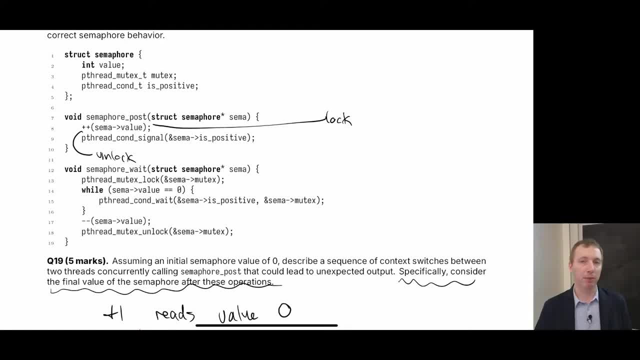 So Remember what the condition variables do. They're basically a way to manage a queue. Signal wakes up The Threads asleep. Signal wakes up one thread in the queue And then The wait function Right. That will atomically. 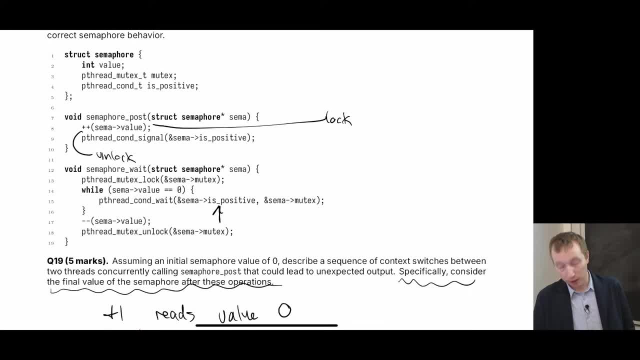 Atomically unlock the mutex and put itself to sleep And then wait for someone to wake it up, In which case, when it's woken up, It will try and reacquire the mutex again. So You have to have the mutex locked. 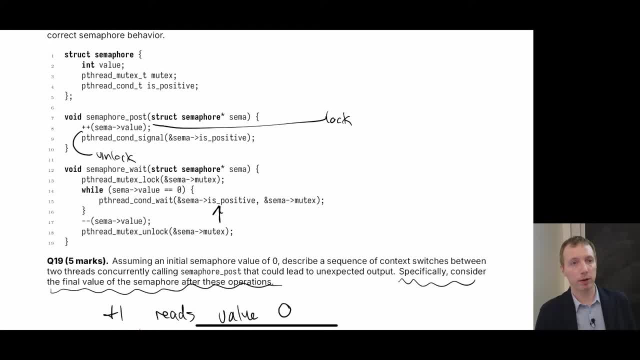 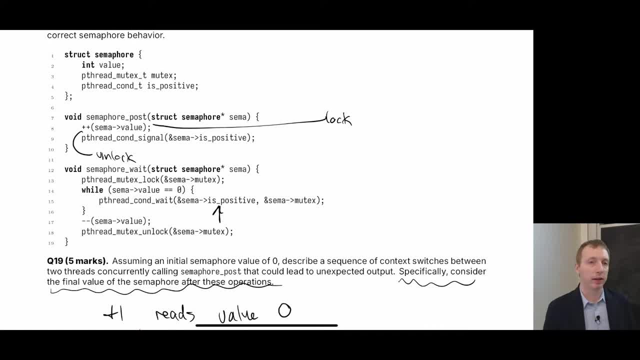 Yeah, Yeah, Yeah, Yeah, And I can do the unlock whenever I want, It doesn't really matter. Um, All right, Oh, That wasn't actually the next question tho. So The next question was: Assume we have two threads, one calling post, one calling wait. 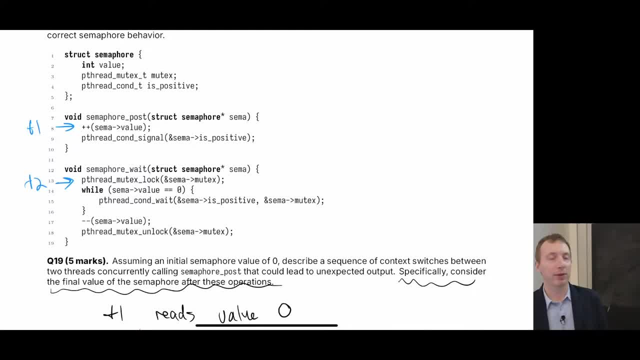 As the code is written. I was nice, even told you what it would be. so I said: is there the case of a lost wake up with this? if so, explain how a lost wake up could occur. so I'll give you a minute to think about that. 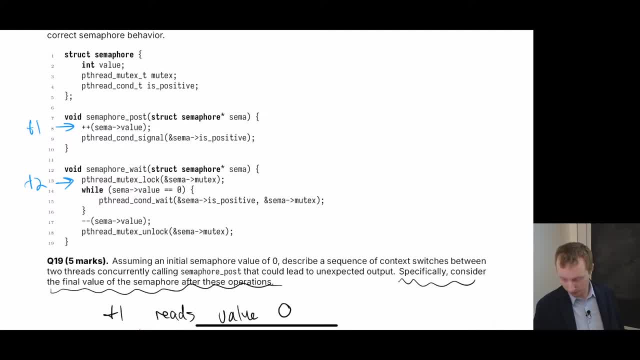 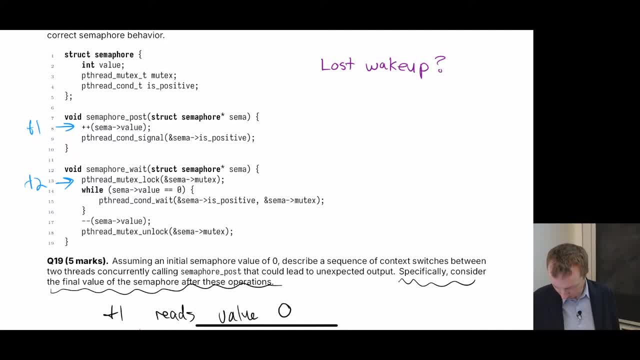 you, you, you, you, No, we have a lost. we should have a lost wake-up right now. Yeah, so the modification should fix the lost wake-up. All right, any brave soul? Yeah, So T2 locks and then enters a while loop so it reads a zero right. 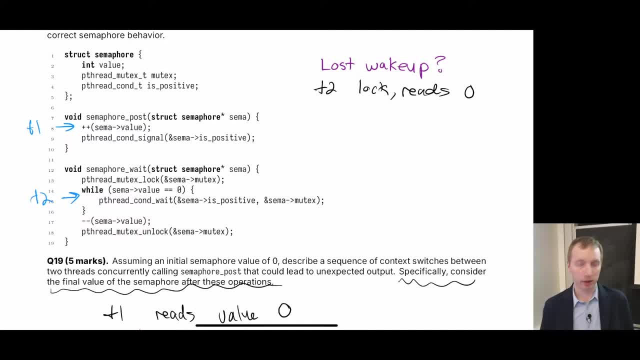 Reads zero. So yeah, it would read a one, write or, sorry, read a zero, write a one. and then it signals Yeah. so it signals nothing happens. now it's done. we context switch back. Then T2 calls wait. 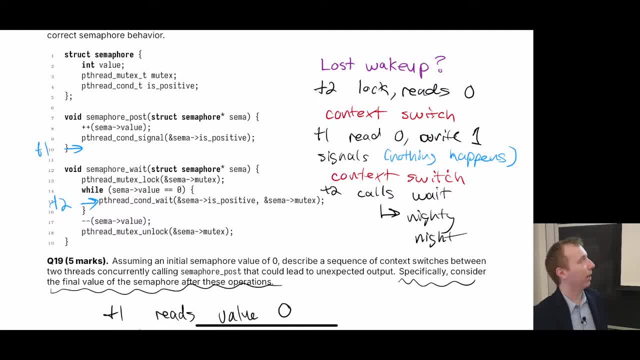 That's The sleep, not going to get woken up again, unless you know something else calls post. But right now the value is one. It should be woken up because, hey, the value is one, now You can decrement it, it's fine, but it doesn't, because we have a lost wake-up. 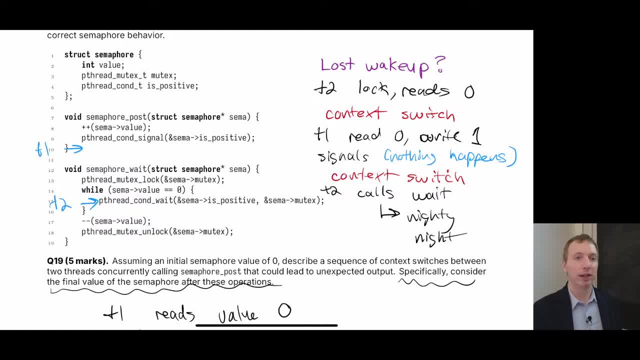 So everyone good with that. Yeah, How, how the wait call is written, It's related to. It's related to the variable that you're passing on to your client. So this is just like the name of the condition variable. So the way I like thinking about that is just like that's the queue. 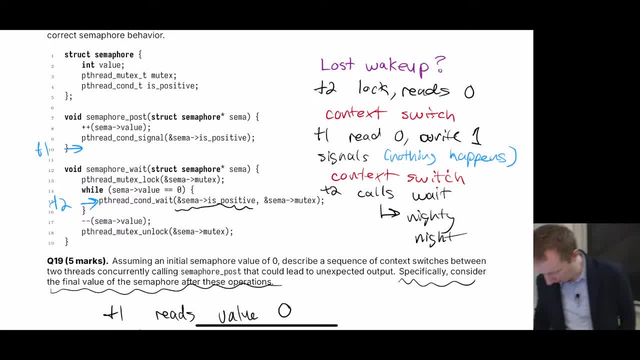 So that's the queue of threads that are waiting, And then the mutex is the mutex that protects the queue and that it reacquires whenever it wakes up. So you know that it doesn't have any data races or anything like that. So 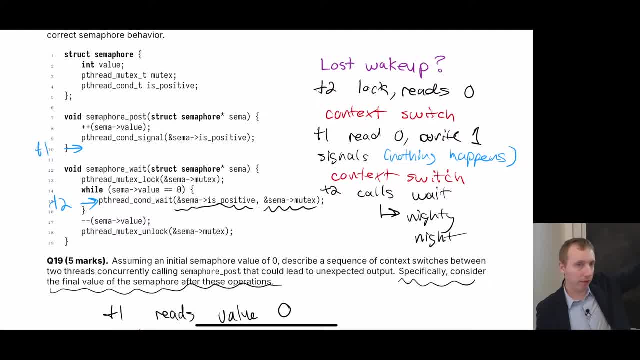 We have the mutex locked whenever we call wait right. In order for another thread to make progress, it has to add itself to the queue. then unlock the mutex while it's asleep so that another thread can make progress And then, whenever someone signals it to wake, wake it up. the first thing it's going to do is try and lock that mutex again so that we don't have any data races or anything like that. 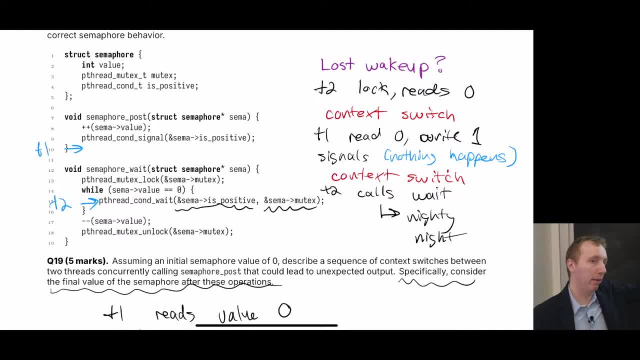 So, because it's next thing it's going to do is read that value again, Right, So we want to make sure we don't have any data Races or anything like that, All right, So, yeah, Next is the fix. So the fix. 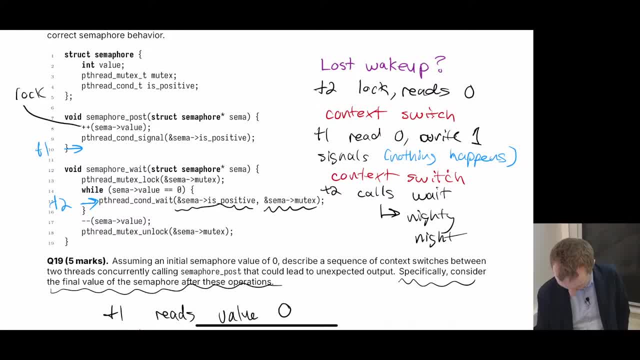 We already said that And then I believe I may have said explain why these things are now impossible. So lost wake up is now impossible because, Well, if we start With thread two, Right, We start with thread two, if we context switch, this cannot happen. 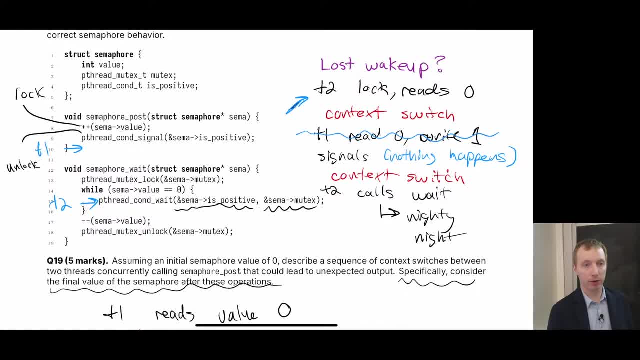 So this cannot happen, because the first thing it's going to try and do is lock the mutex Right. So this can no longer happen anymore. So even if we context switch, nothing is allowed to happen. So it can't make any any progress. so we have to switch back to thread two to make progress. then it 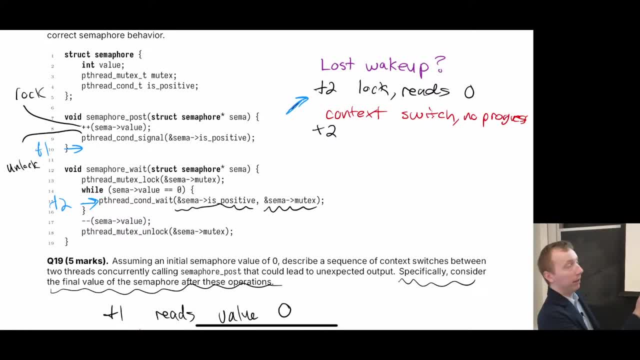 would. after reads the zero, then it waits, so after wait, so I can draw, like the queue up here. so initially it's empty. when it calls wait, then what it will atomically do is add itself to the queue. was that we called it thread two and then unlock? 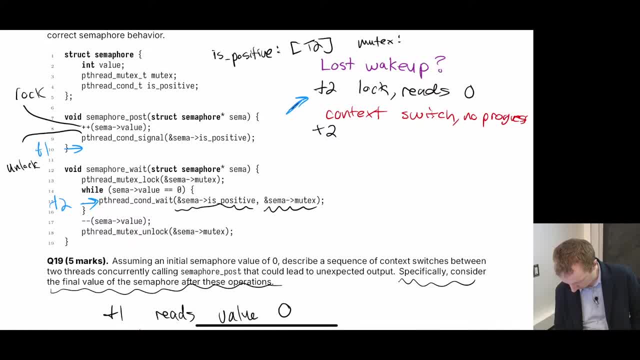 the mutex. so I could just say mutex is now unlocked, right, so now thread two is asleep. the mutex is unlocked. the only thing we can do is we can context switch back to the queue and then it will add itself to the queue and then it will just say mutex is now unlocked, and then it will add itself to the queue and then 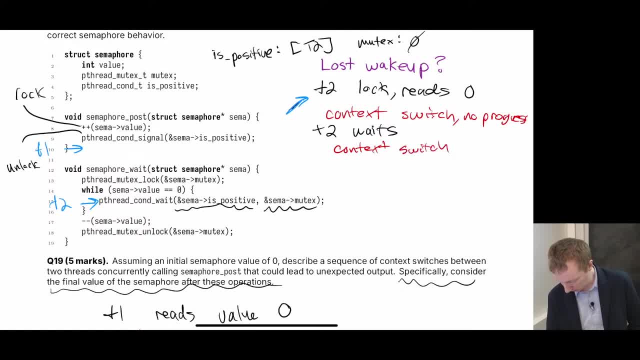 back to thread one. well, then it could go ahead. whoops, thread one could lock. then it would update the value from a 0 to a 1. so I'll just shortcut it and just say: writes a 1 and then right now still nothing else can run. only thread one is. 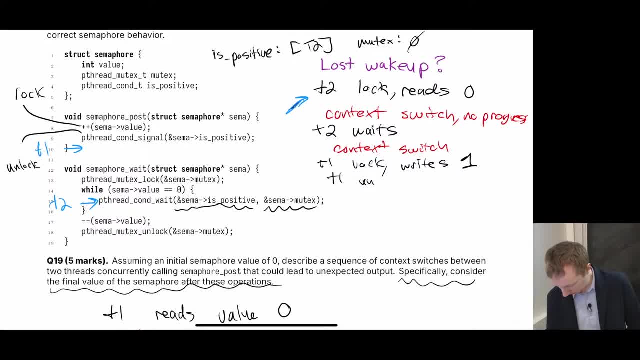 allowed to run, then thread one unlocks. as soon as thread one unlocks, then it signals. so now it no longer has the mutex. oh whoops, I should have written here: so thread one did have the mutex, now it doesn't. now it unlocks and then it signals. so now thread two can go ahead and execute before returning from that wait. 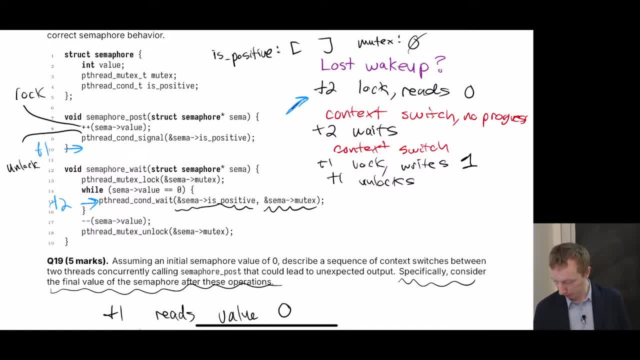 call: it needs to reacquire the lock so I could context switch over to thread context switch back over to thread two. it reacquires the lock because no one has it. it now it парfolios with stringer. what if no one has saved me? and now? 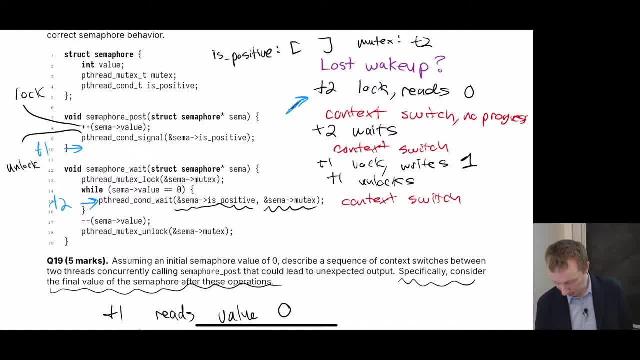 it would go ahead- and that's why we had the wow. so it would go read that value again. now the value does not equals 0, so it would go ahead and pass and then decrement the value from a well, from a one to a zero, and we're all. 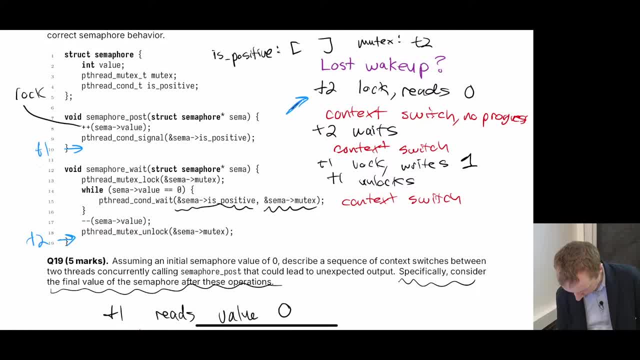 good, now it unlocks the mutex, and then we're done so after. so this is what you suggested, right? so let's see what happens there. so let's rewind. so all right, so let us rewind a little bit. so right now, thread two is in the queue. it has hit this weight. 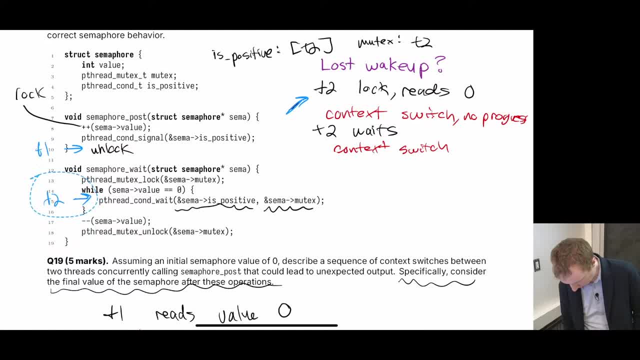 so it has hit this weight, so no one has the mutex anymore. it is now asleep and we're context switching back over to thread one, right, something like that. so now what might happen is okay, well, thread one locks rights of one and then signals: right. so if it signals now, thread two is out of the queue. could. 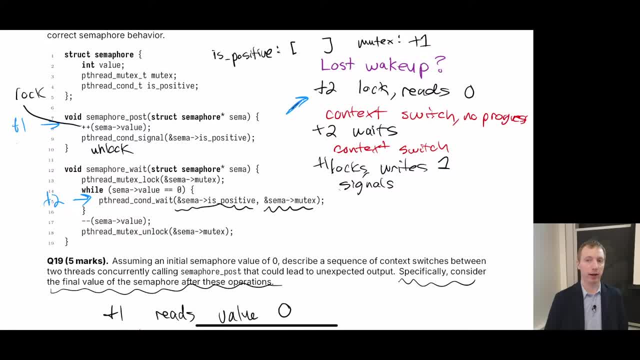 run and now thread one has the mutex right. so what could happen right now is we context switch. oops this, I don't know why this isn't blue, so now we context switch. so if we context switch to thread two right now, can it a turn from the wait? No, why? Yeah, thread one has the mutex right, So it's woken up and it's. 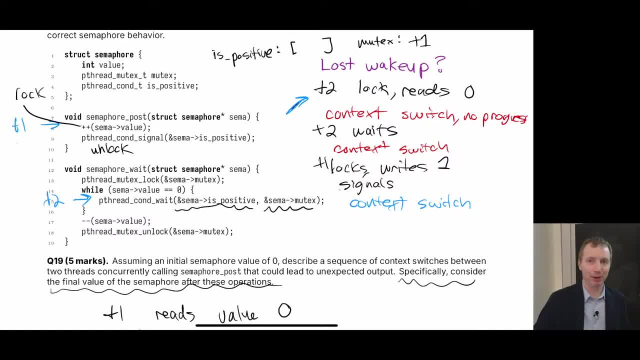 not going to be able to get the mutex. So technically, if you really really really care about like micro-optimizations, you should have the unlock first and then the signal, but it's not going to affect like the correctness at all. This might be a bit slower because now 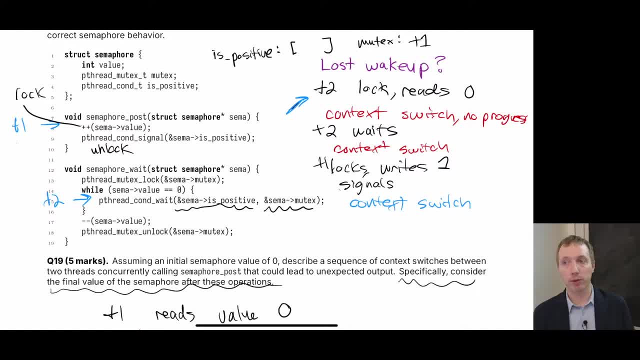 we can context switch to thread two. Thread two would try and acquire the mutex. It can't because thread one has it, So we have to context switch back to thread one. So when that happens, essentially it tries to acquire the mutex and essentially it just waits. 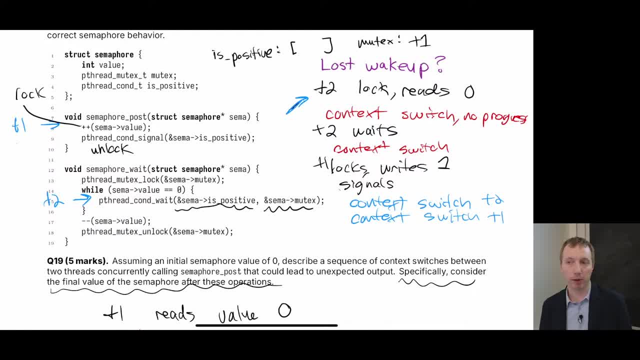 on the mutex. Yeah, so it would try and lock the mutex again and then it would go into like the mutex queue Instead of that, like a condition variable is basically a queue we can manage, but the mutex would also have its own queue. So there's queues on queues, and which is great because we love. 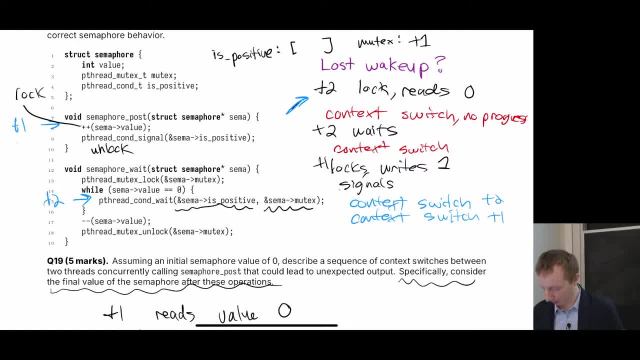 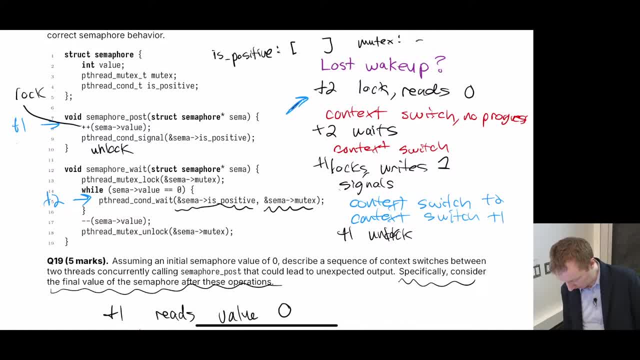 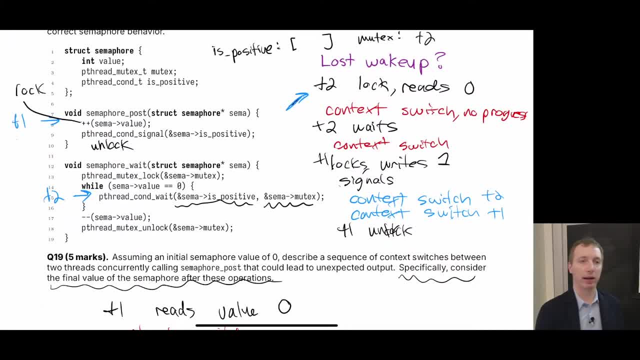 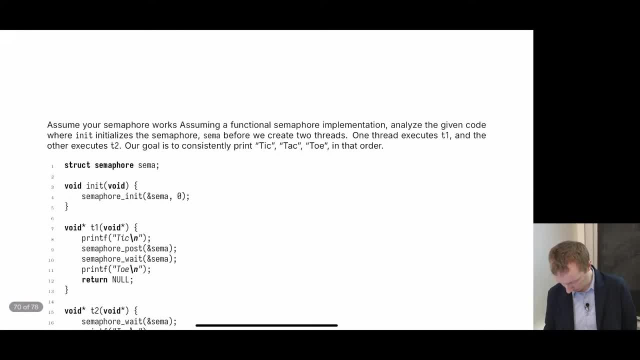 All right, Any other questions about that one? I think that covered everything and we got a little bonus, So that's good, That's good, Oh, okay, Here's a fun question. We should have more than enough time for it. 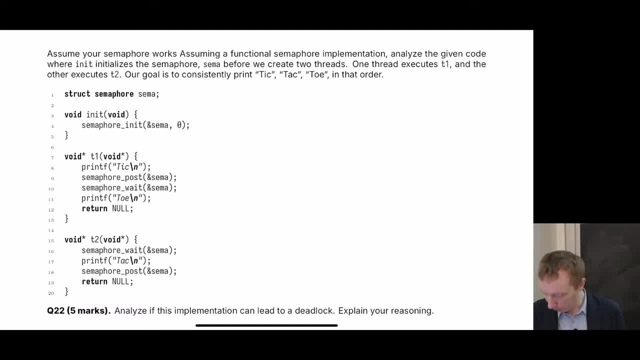 So this now says: assume your center for works, assuming a functional center for analyze a given code where it initializes a center for. So right, here we initialize the value to be zero And then we create two threads, So thread one executes one thread. Here I'll call it something nicer. 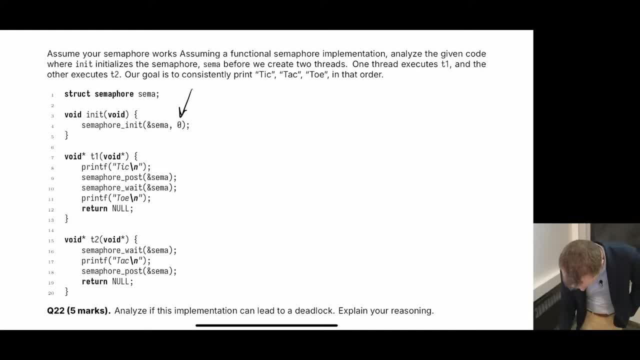 Here, I'll call it something nicer. So thread one wants to execute this function, and then we have thread two that wants to execute this function. So our goal is: we always want to print tic-tac-toe and always want to do it in that order. 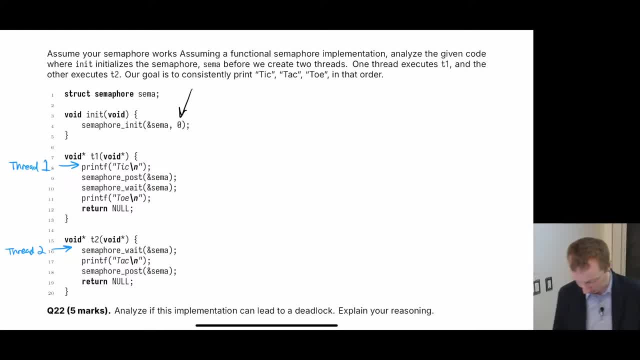 We're not allowed to move the printf statements between the threads or anything like that. So first question is: analyze if this implementation can lead to a deadlock, And that's like a deadlock in any thread, like: can any thread be stuck where it can't make any progress? 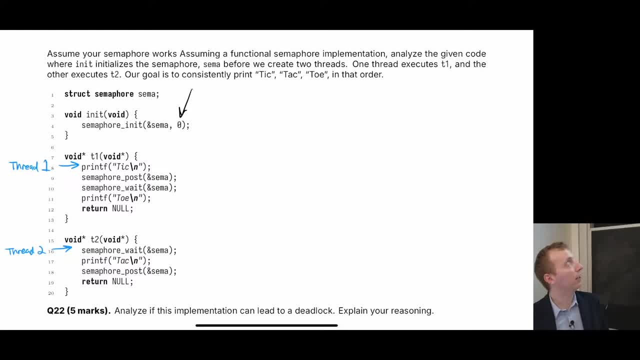 Yeah, Yeah, So it can. Yeah, So what may happen is thread one. so here's our center for value. I'll just write it over here. So currently the value is zero, right? What could happen is thread one executes, we post. so now the value is one, and it would do that atomically. 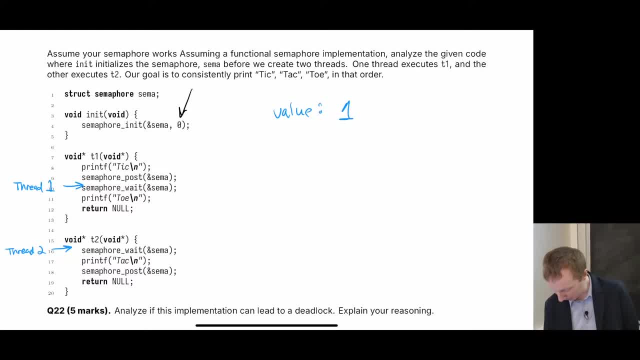 Then well, thread one can continue executing and call wait, Then wait would update that value from a one to a zero, Then it would print toe, so we would see tic-toe. And now if we switch back To thread two, it's at a wait. the value is zero. it will never change, right. 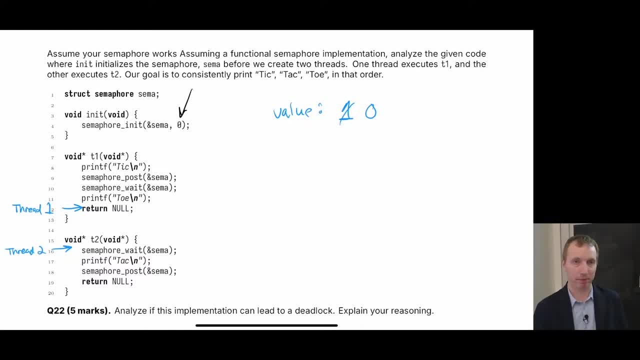 Now it's stuck, Thread two gets deadlocked, So can't make any progress anymore. So there is a case where it would, because ideally what we want to happen, and if you actually run this, it will generally actually print tic-tac-toe most of the time. 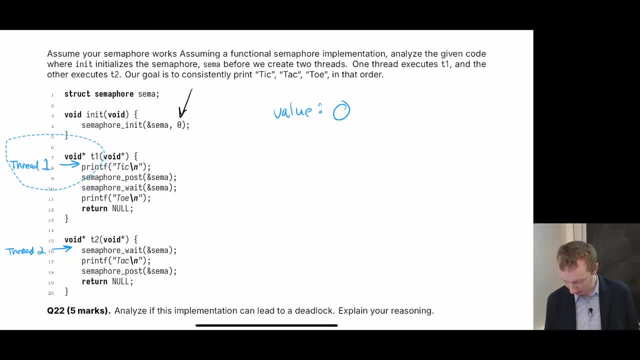 Because what we were thinking is: well, we print, tick, then we post, right, so we change the value from a zero to a one, and now we want to context, switch to thread two, then thread two- can you know, wait? change the value from a one to a zero. then print, tack, and right now, if we 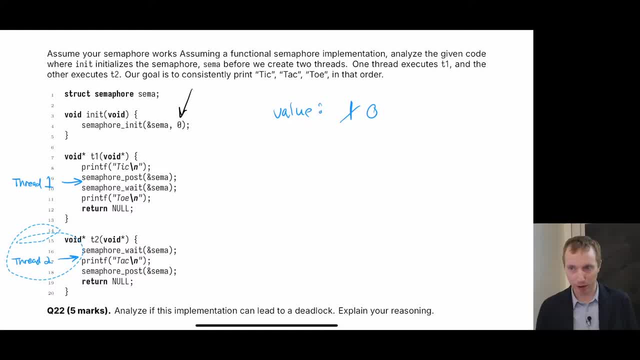 context, switch to thread one. thread one can't make any progress, then we would post whenever after we done, after we are done printing tack, update that value from a zero to a one, then thread two can go, or thread one can go ahead, pass this weight and then tow, and then it's in the correct order. but yeah, what might happen? 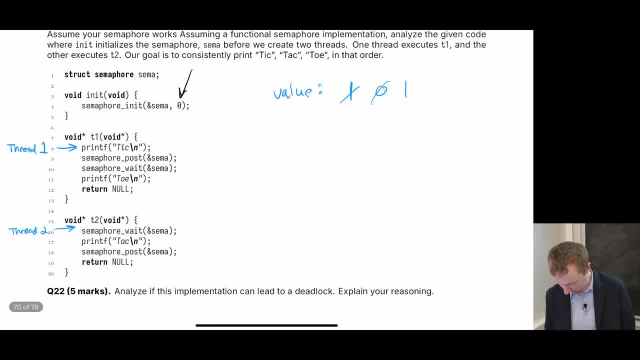 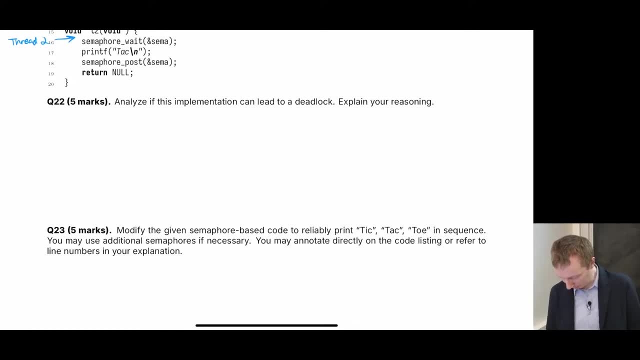 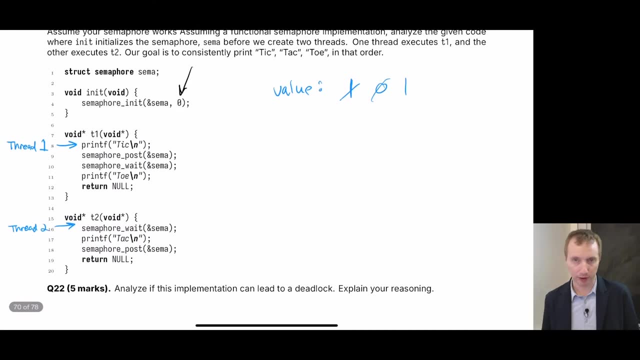 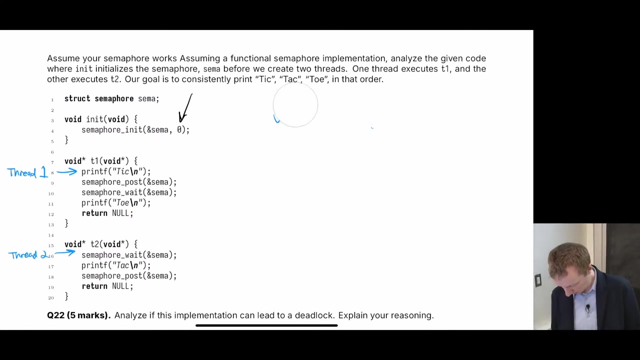 is it deadlocks, or at least one thread gets stuck. oh, and then next question was: modify it so that it is correct. you can use additional center force if you want. go ahead directly, annotate the code if you want, and refer, just describe it and refer to line numbers. so yeah, and 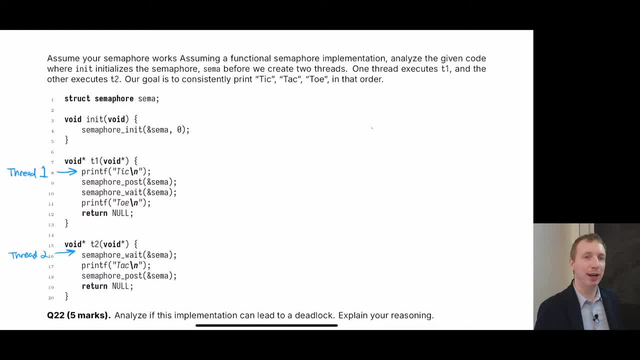 spoiler alert: this question came up because someone asked: hey, can I just use one center for for something like this? and then also we had a foster dog that was named. what was her name? tack, because they were three of them and they were tic-tac-toe. so I merged both of. 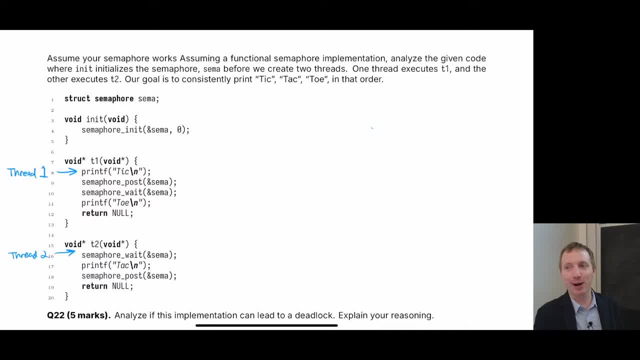 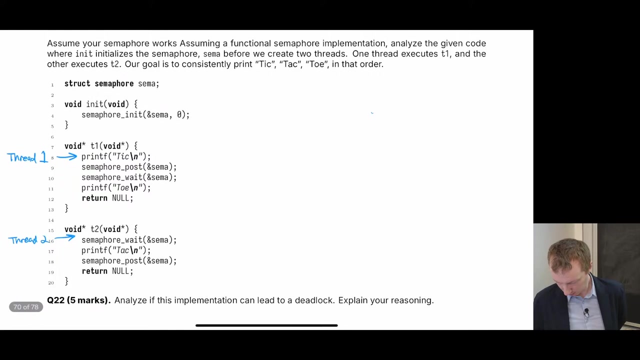 the ideas and boom. if you ever want to know how I come up with questions, it's purely random, all right. so give you a minute to think about how we would fix this, yeah, or we'll wait. you, you, you, you, all right, any solutions? all right, any solutions. 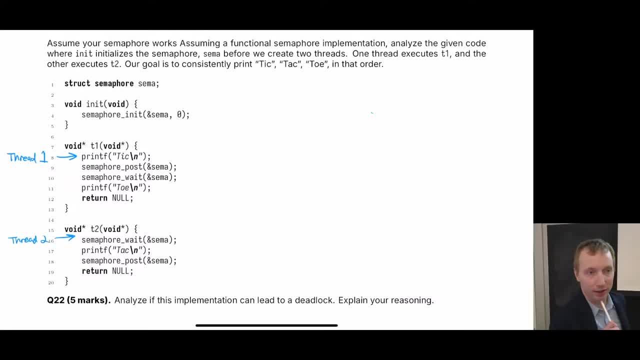 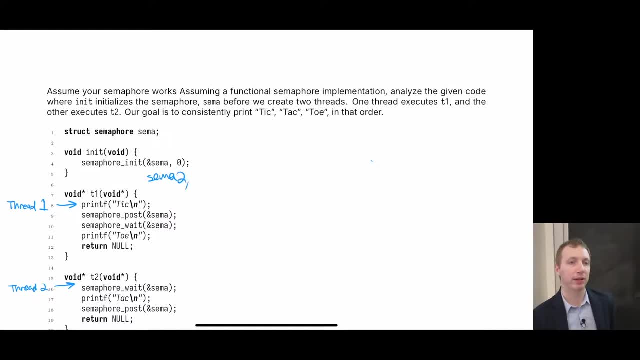 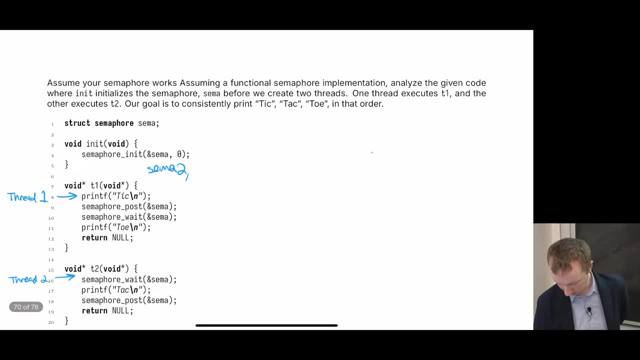 Yeah, so I need two center fours. so I'll create another one sem of two, So they both weight on different center fours. So this should be, I'll put it, I'll make that better. So this should be sem two, okay. 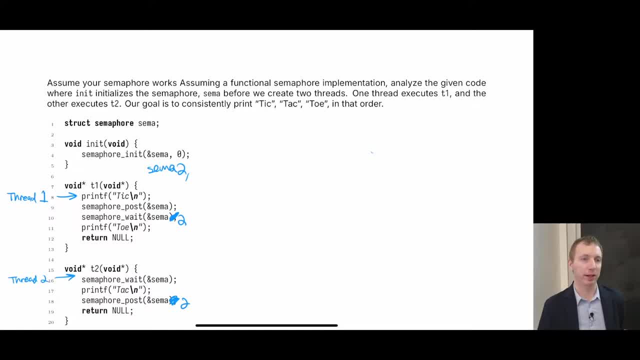 So this should be. and then what? should the initial value of the center four be Zero? boom. So there's our fix. So that should work now. So now, if thread two is waiting on whoops, If thread two is waiting on the first center four, it can't make any progress, right. 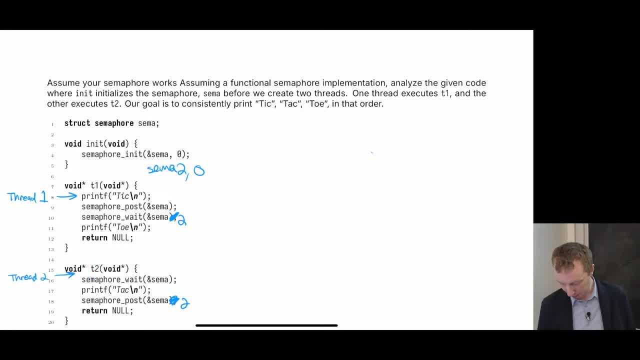 The value is currently zero So it's stuck, can't make any progress. Thread one has to run print tack and then it would post sem like the first center four So it would increment it and now it can't make it past this because its value is zero. 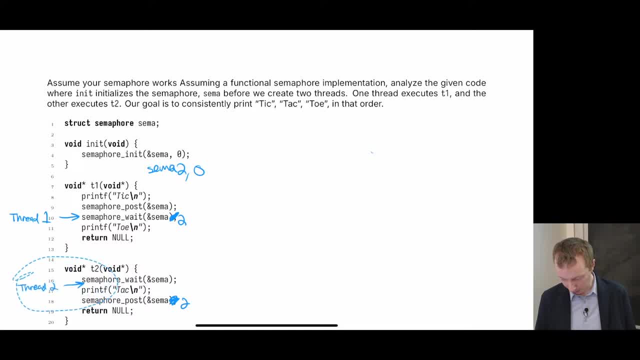 So thread two is the only thing that could run. It could make it by the weight Print tack. and then, well, if we switch back to thread one, still can't make any progress because the value is still zero. Now thread two can go ahead. post the other center four changes its value from a zero. 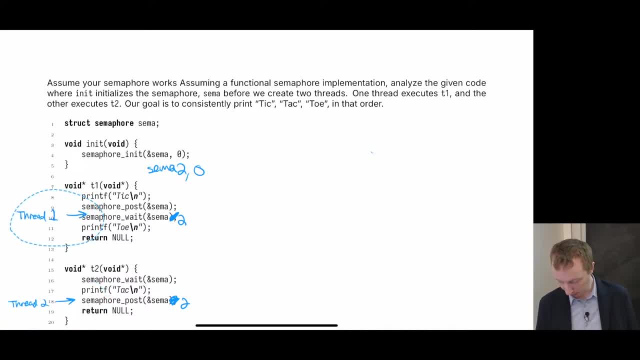 to a one, Then thread one can actually pass this line and then we get tow, so we get tic-tac-toe Cool. All right, all good with that question. All right, seven minutes. Should we try and speed run a question? 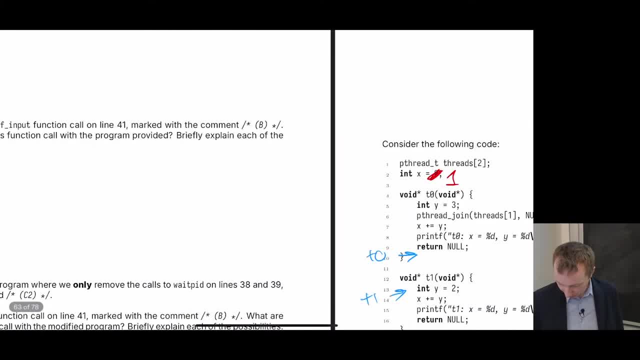 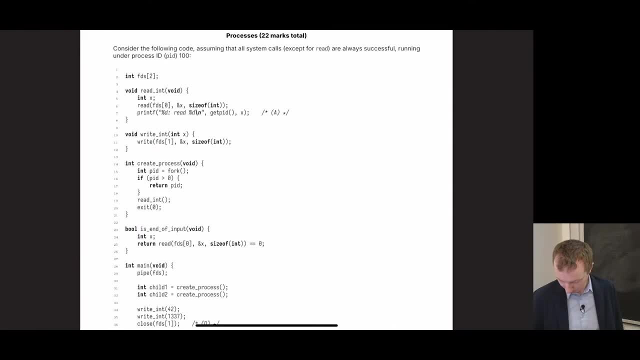 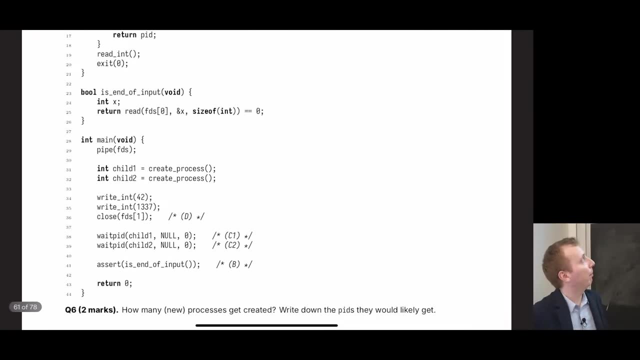 All right, let's try. So other one that is hard. The other one that is hard is probably this process one. So this process one was: I'll just try and describe what it actually does and then, hopefully, you can answer the questions. 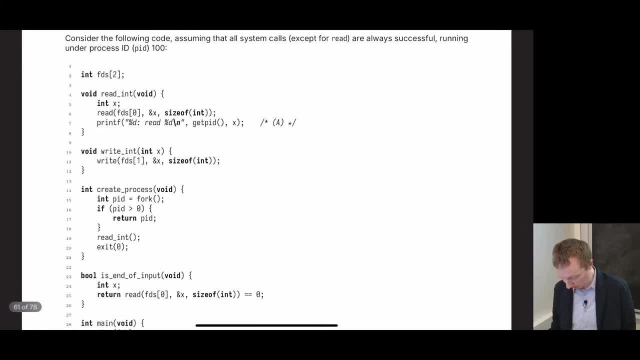 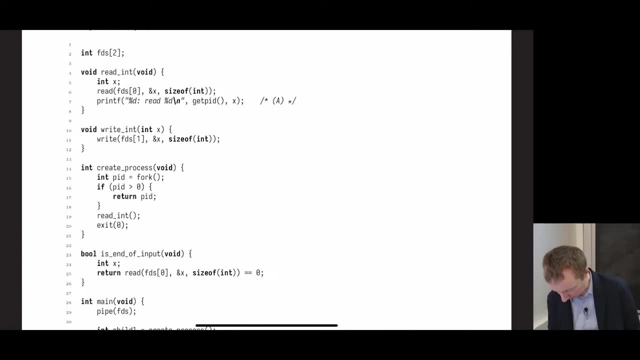 So this one was a little bit more involved because it actually tested some file system stuff too. So what this does is There is a global variable called init FDs, because we're going to call, pipe on it and then share it between all the processes. 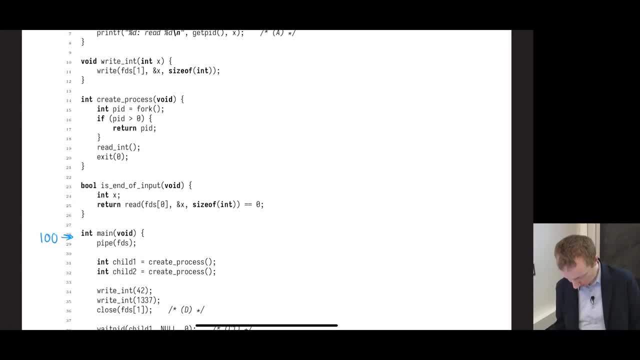 So we have process 100 here It calls pipe. So we make a pipe with FDs, We assume it's successful all the time, so that we have a read end and a write end, and then we create two processes. So here, 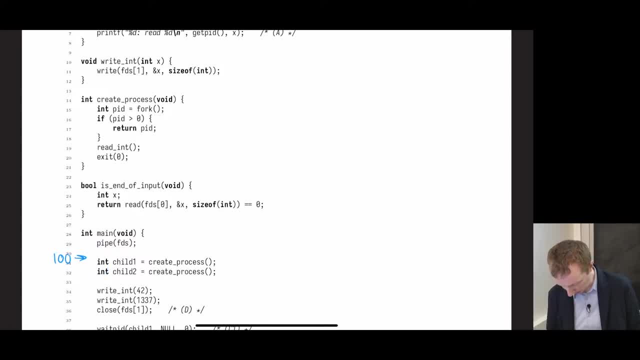 Let's assume that child one and in the create process what it does- I was nice- We fork. Then we don't know which one is going to run. Assume we have processes 100,, 101, and 102. So if PID is greater than zero, that means we are the parent. 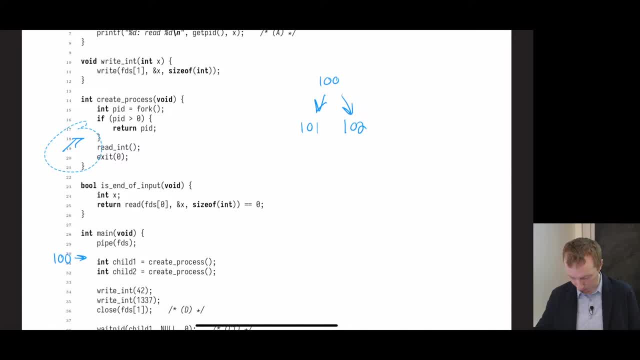 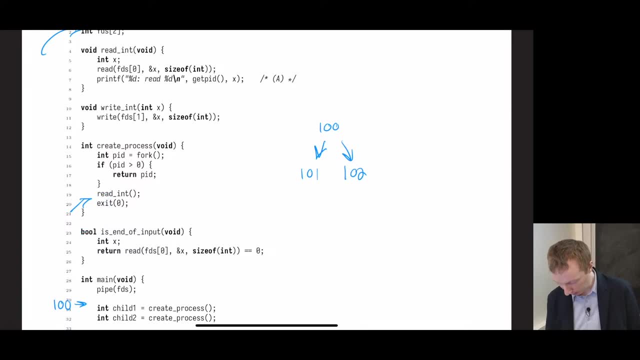 I just return the PID. So we get the PID returned And then all the child does is call read int, which all read int does is read an integer from the read end of the pipe, And that's all it does, And then it exits. 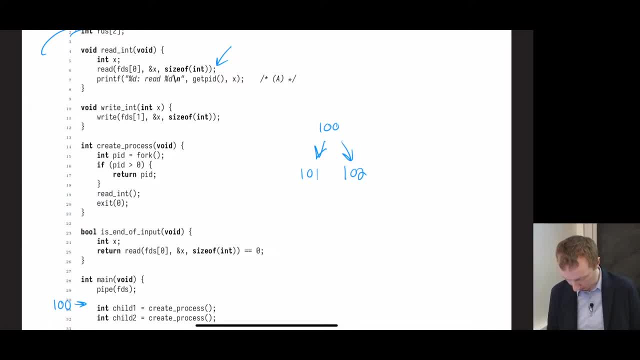 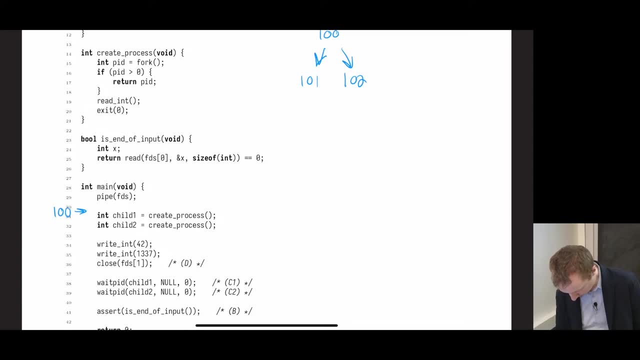 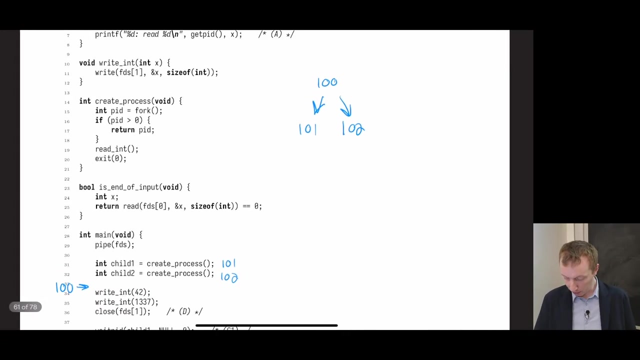 So the child children don't really do anything that involved. So it would just look like this: So we get 101, probably 102.. That's the two return values in our parent process. Then our parent just writes- Right now we don't know what order things would run. 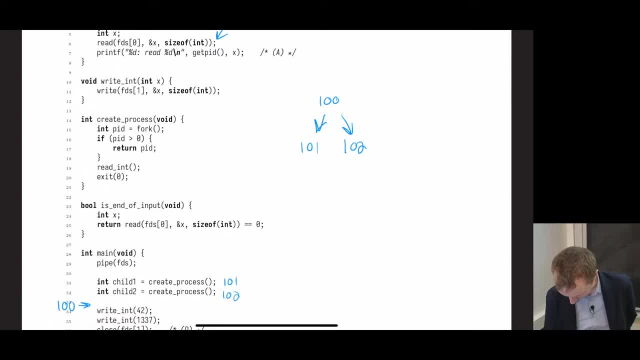 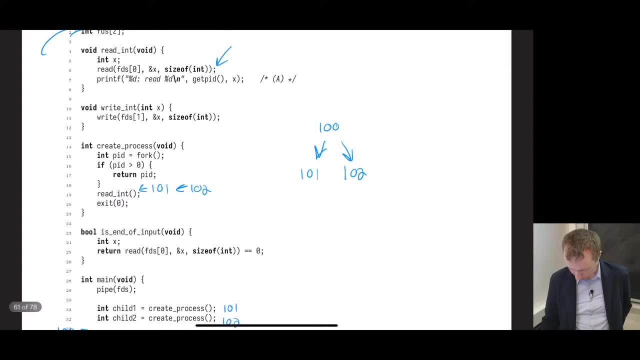 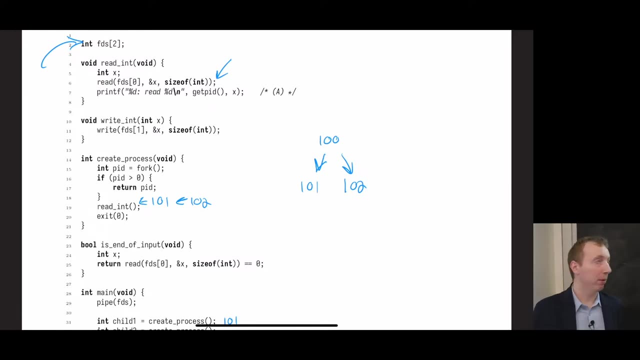 If right now the child ran, so let's say they were both here. they call read int, which reads from the read end of the pipe. Currently there's no data in the pipe, right? So read is a blocking system call. We'll just sit there and wait forever until we actually write to them, right? 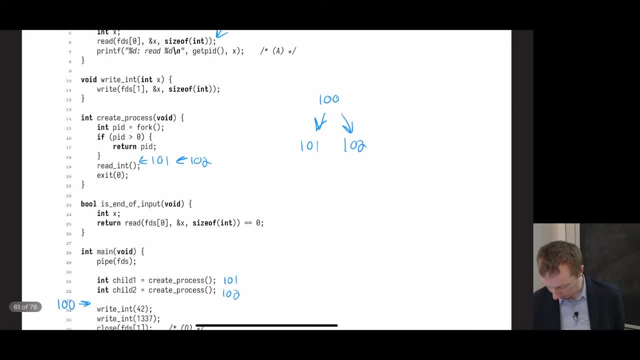 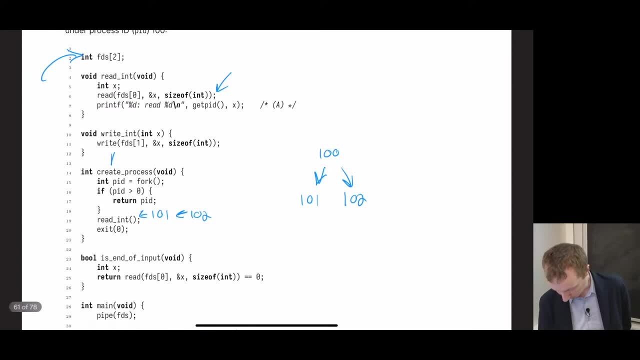 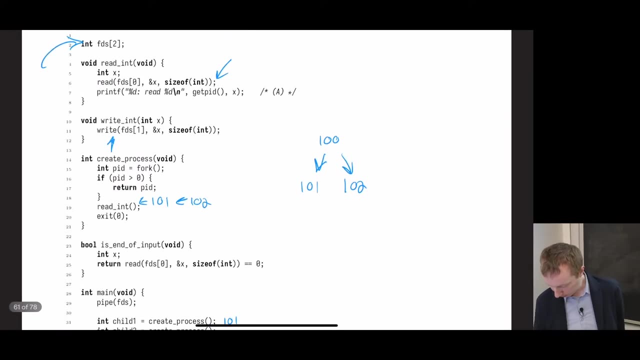 We don't know which one's going to execute. We don't know anything about that. Then eventually the parent process is going to call write int, And what write int does is just write an integer to the right end of the pipe. So now it writes the number 42 to the right end of the pipe. 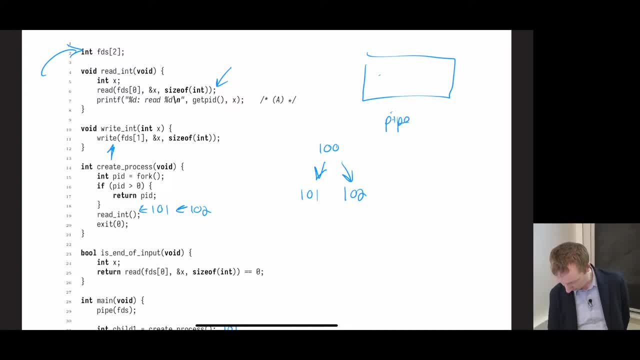 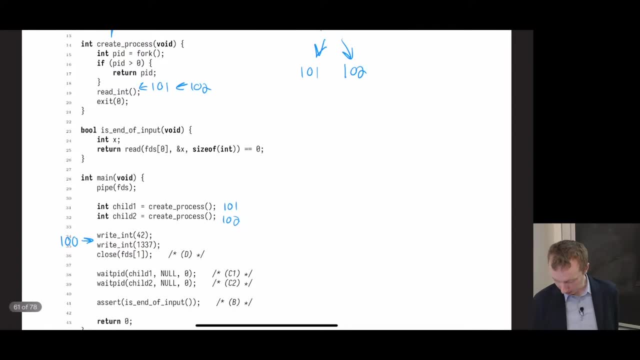 So here is our fun pipe. So it puts like a 42 in there. Now We don't know who's going to run next. Maybe it writes, Maybe it writes 1337 next and there's two numbers in the pipe. Don't know. 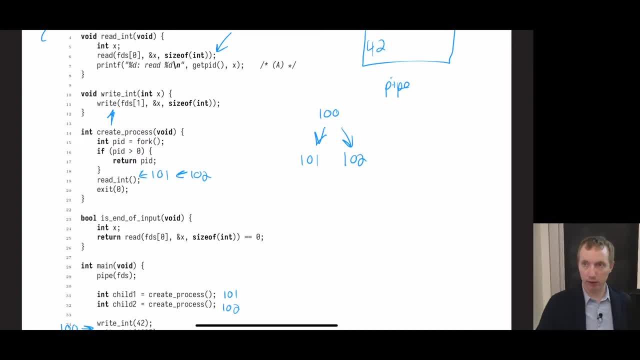 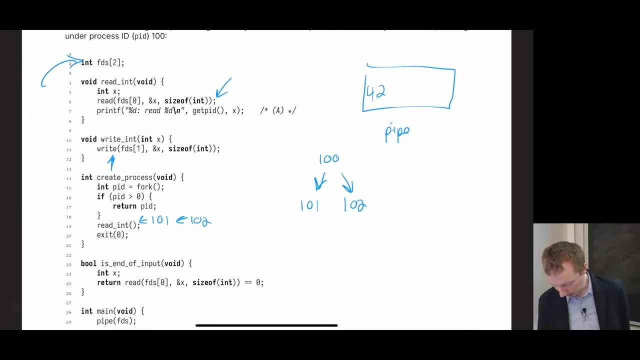 Maybe process 101 executes next and reads an integer in the pipe. Don't know, Maybe it's 102.. Don't know. So anything could possibly happen. What could happen is, let's say 102 could read. Now it would read 42.. 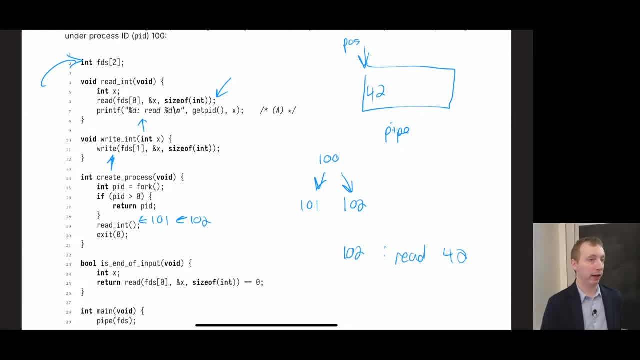 And because there's like a position in the buffer and since everything's shared in that global open file table, after it reads that, it would advance the position to here: Whoops, Move, Okay, Moving too much. Advance the position to here. 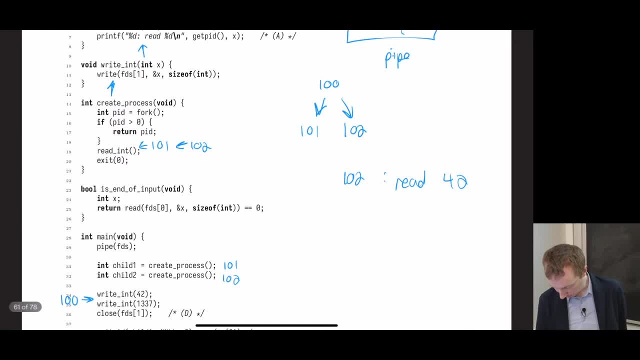 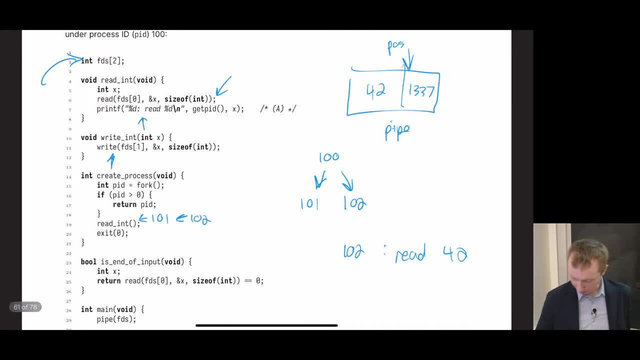 And now, well, process 100 could go ahead and write 1337.. Okay, 1337 to the pipe. Now, if process 101 wakes up, it could go ahead and read 1337.. And now they're done, And there's no way that I can possibly read 42 twice because, well, everything got forked. 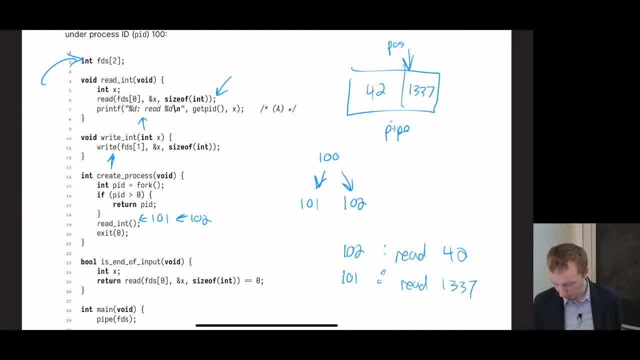 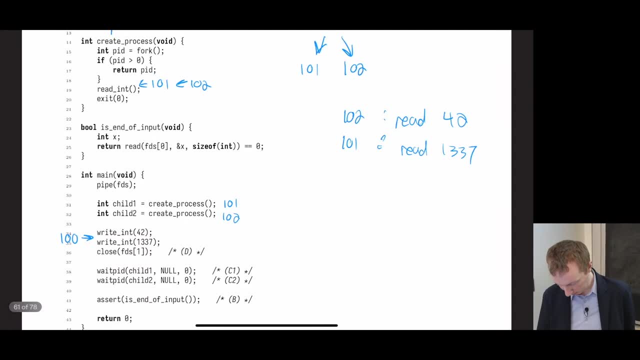 together. It's the same global open entry. They share the same position, They share the same everything. So we won't read the same number twice. So that is one possibility We might have. And then process 100 closes the right end of the pipe, so that you know we can actually. 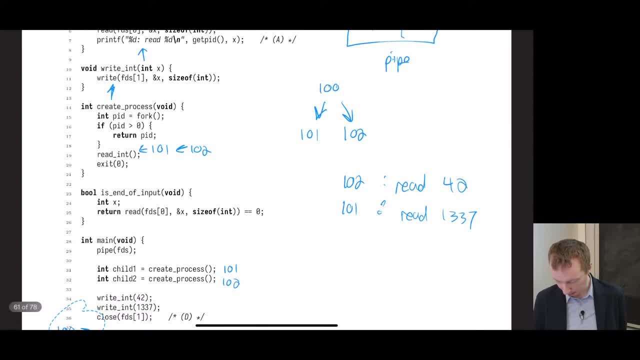 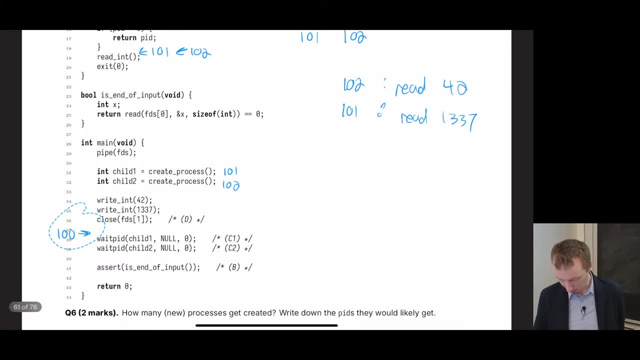 know that no data is possible. So after they read then they'll exit and then close all their file descriptors And then process 100 would be the only one with a right end of the pipe open If it closes it and then waits for the child. 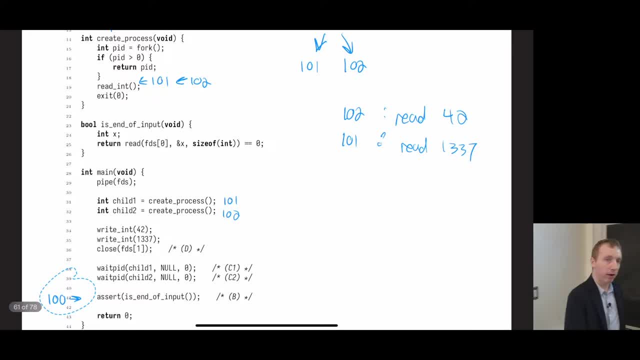 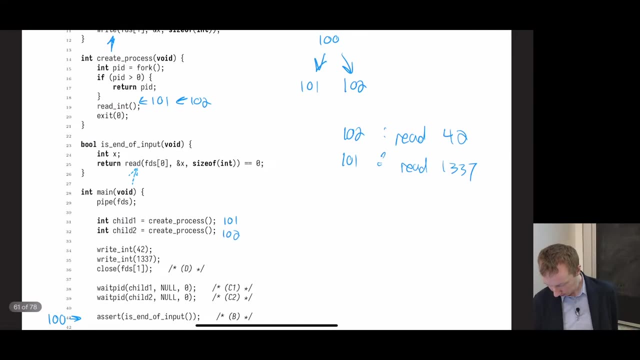 Then whenever it calls end of output, Then all of the right ends are closed, So there's no possibility for some output. So read will just return zero, And then we would get end of output returns true, And then we're done, Right. 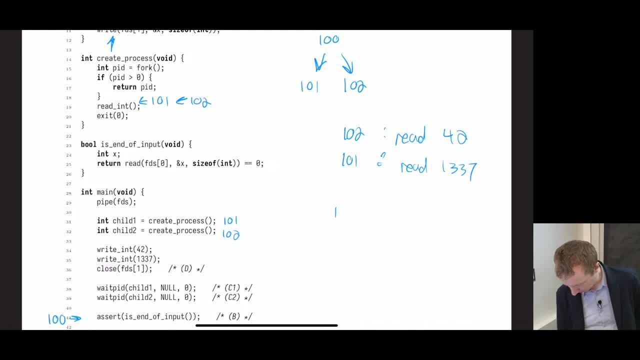 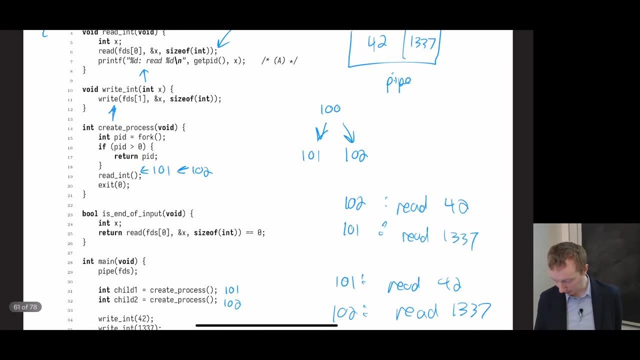 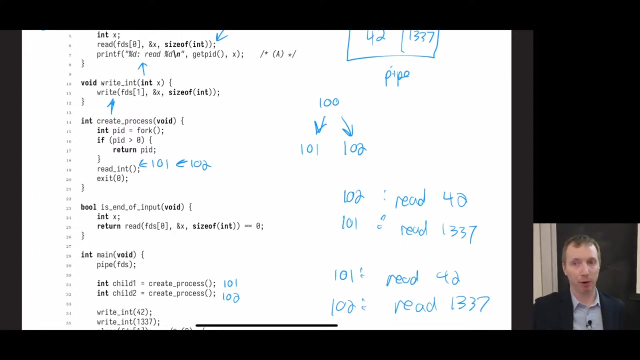 And other possibilities are well, process 101 could have read 42 first. Process 102 could have read 1337 after Right, Okay And other possible outputs is well, maybe process 102 read 42. But it got context switched before printed. 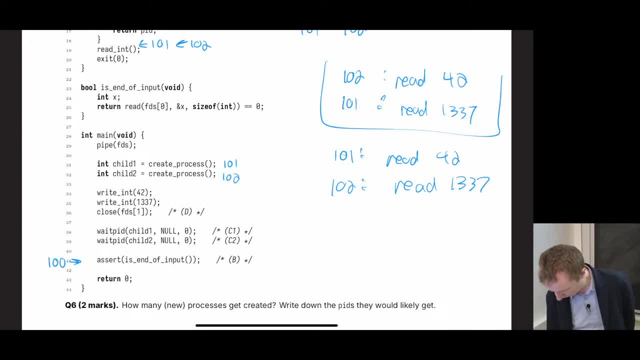 So another possibility is just like essentially this, with what they read, but in the other order. So we could get 101 printing off 1337 first, This printing off 42. Or similarly I could do the other order of this. 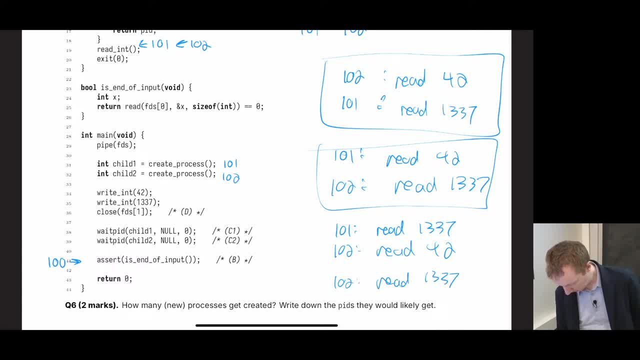 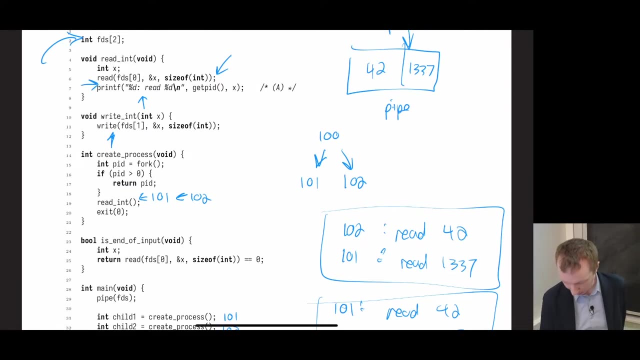 So 102 could read And then 101 reads 42. And this is where they get context switched like fairly suddenly. So they get context switched right after they read and before they print. So I made that worth less Yeah. 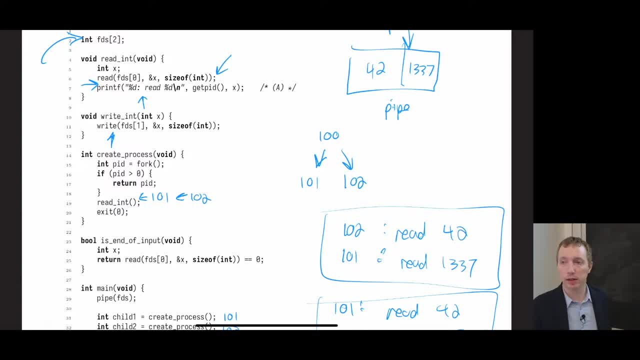 You mentioned that the right ends of the pipe, Like now that we have right end of the pipe So we could get context switched right after they read and before they print. So I made that worth less. Yeah, But when you close the right end of the pipe and the current, doesn't that still reopen? 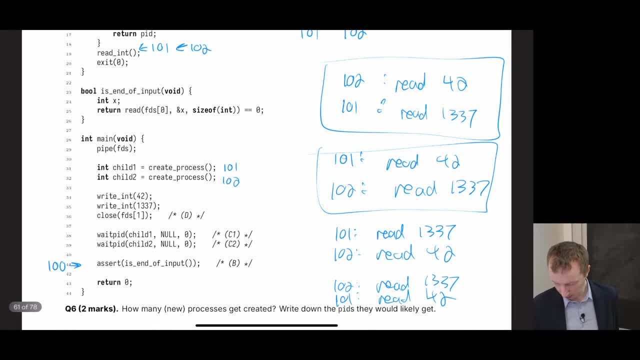 the children: Yeah, But I also wait for the children here to finish, Yeah. And then one of the questions you can read on is like: what happens when I remove this? Then I think the other one is: like what happens if I remove this? 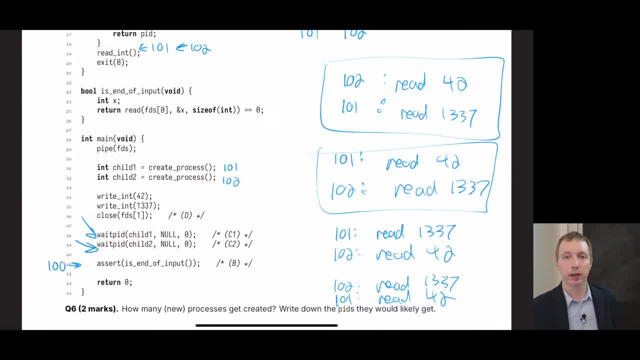 And then like, does this always print? And you can go through that, But hey, we're out of time now, So thanks for sticking with me the whole time. I'll see you next time. Bye, Bye, Bye. 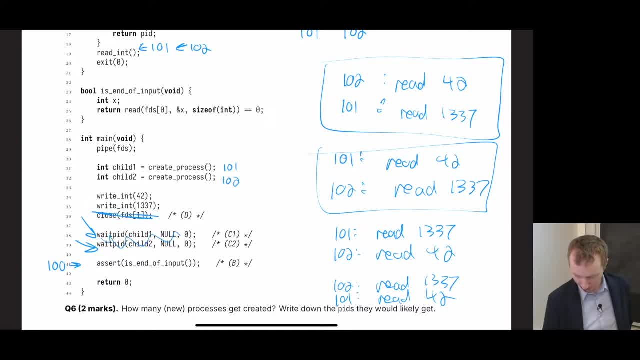